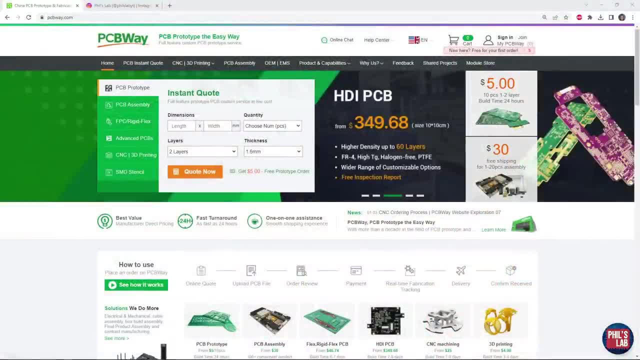 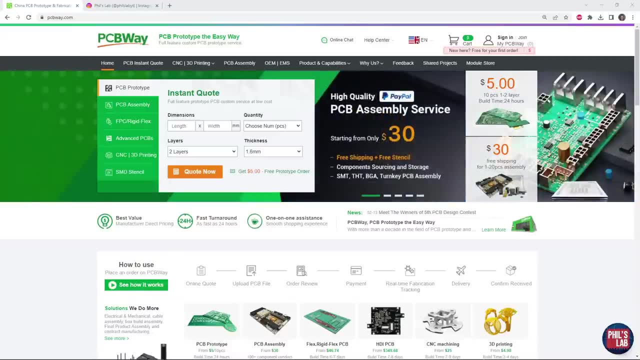 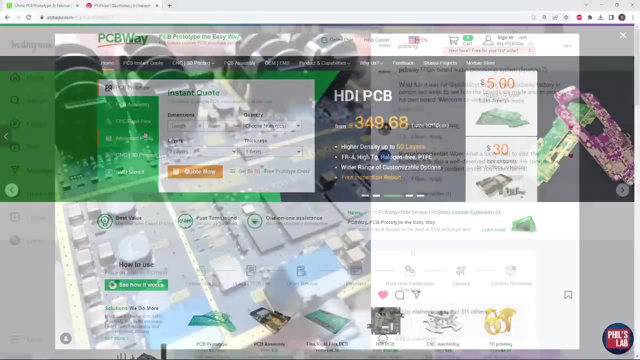 A huge thank you also to PCBWay for sponsoring this video. The Xerxes PCBs were manufactured and assembled by PCBWay and they did a great job assembling small O2O1 components, BGA packages and an Impedance Controlled 6-layer board. For this I used their Advanced PCB Design service. 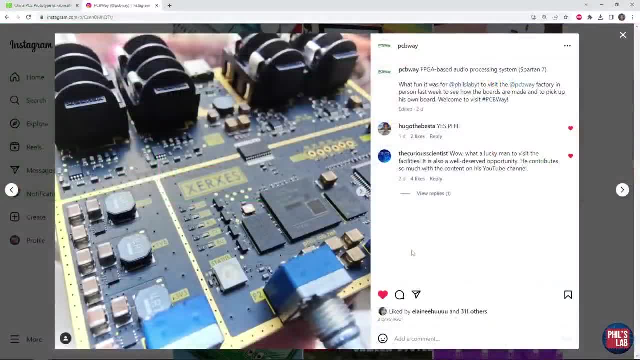 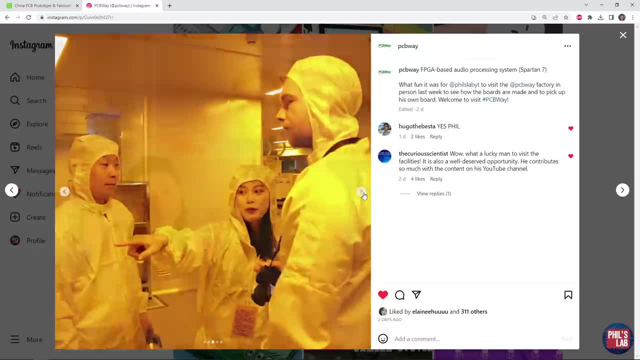 The cool thing is I actually picked up these boards personally from PCBWay as I visited their Shenzhen factories last week, and I recorded a video of the whole PCB manufacturing and assembly process. So thanks again for PCBWay for such a cool experience. I also have a new course out. 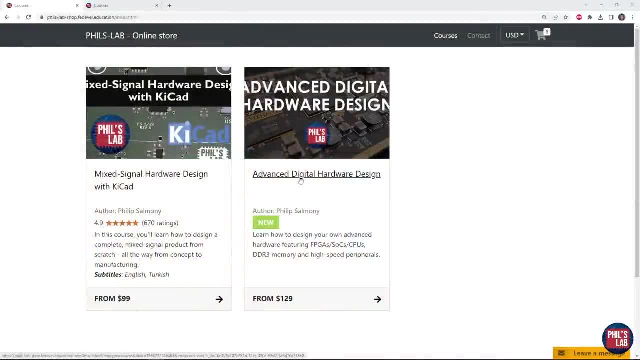 called the Advanced Digital Hardware Design course, where you can learn how to design your advanced hardware featuring FPGAs, system-on-chips, high-speed DDR3 memory and high-speed peripherals with Ethernet and so on. I'll leave a link to this, as well as the course content description. 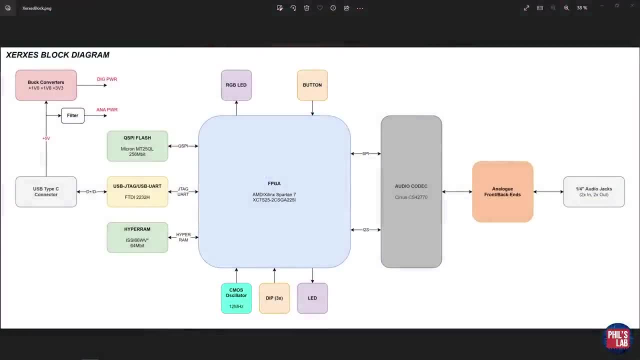 in the links below this video. This is the block diagram of the Xerxes PCB. you saw at the beginning of this video. The main purpose of this board is for digital signal processing of audio signals, and we'll see more of this in future videos. In this video, however, I'd like to show you the very 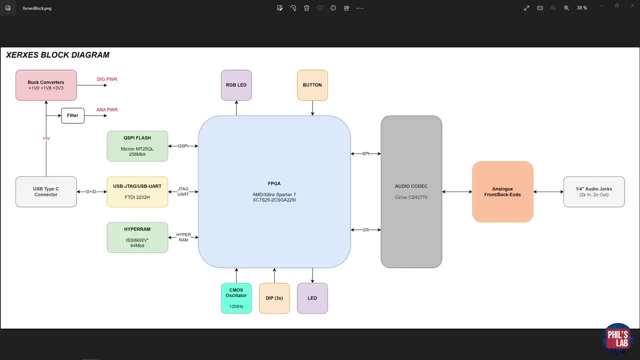 basics of writing some Verilog HDL, getting an LED to blink, reading DIP switches, and how to program the device and do the whole project setup, all the way from an empty project to actually writing to the configuration memory. I feel like a lot of tutorials that are online show you how. 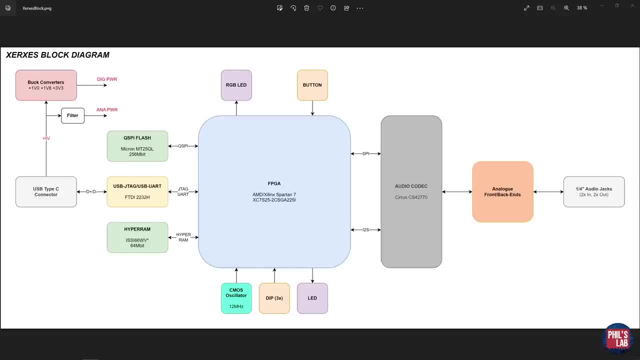 to do this with a pre-made board where you have all the files already set up for you and doesn't actually show you the whole process. so that's what I'd like to do in this video. We'll only be using a few of the parts shown in this block diagram, in particular the centerpiece, which is 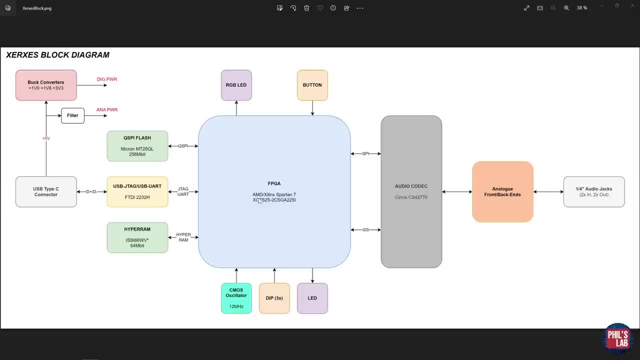 the FPGA itself, which is an AMD Xilinx Spartan 7.. Connected to that is a USB to JTAG and USB to UART converter through which we can program this device very easily without needing an external debug probe, for example. This then feeds to a USB type C connector, through which the board is. 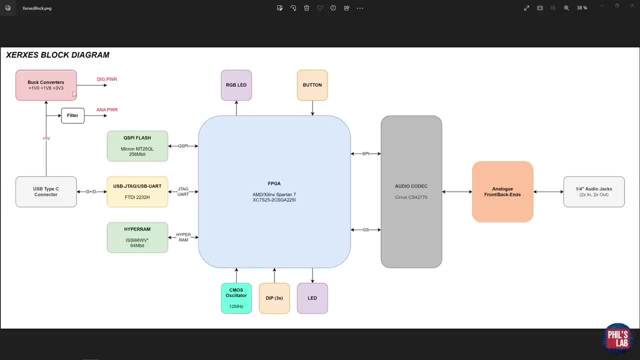 also powered from 5 volts, feeds, various regulators to feed the analog and digital sections. What else we need to know is that we have a CMOS oscillator, so a clock input at 12 megahertz. we have three DIP switches. we'll be using one of those DIP switches, as well as an LED which we can toggle. 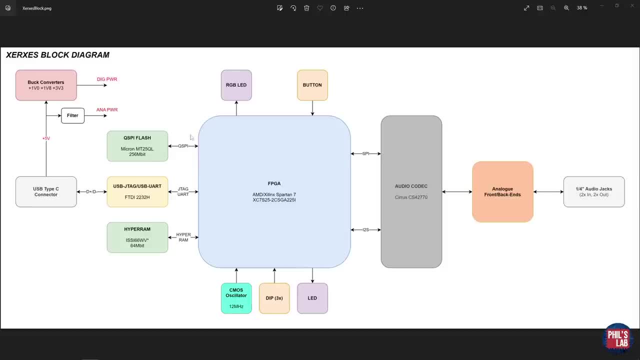 on or off. Later on we'll see. we also have some QSPI flash memory, which is the configuration memory. for example, during boot up of our board, the FPGA can query the QSPI flash memory and then pull in the bitstream to reprogram the FPGA itself and then load our HDL onto it. We'll see how to do. 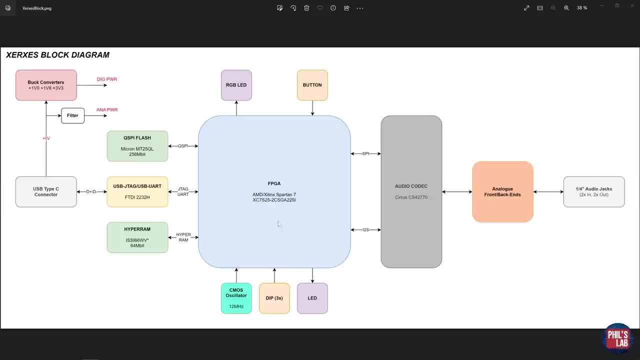 this later on in the video, But for now, let's get started with creating a project and setting up our blinky code. In essence, we'll be flashing the LED at a certain rate, with a certain on and off time, and we can control the speed or the frequency or the length of the on and off time using one of 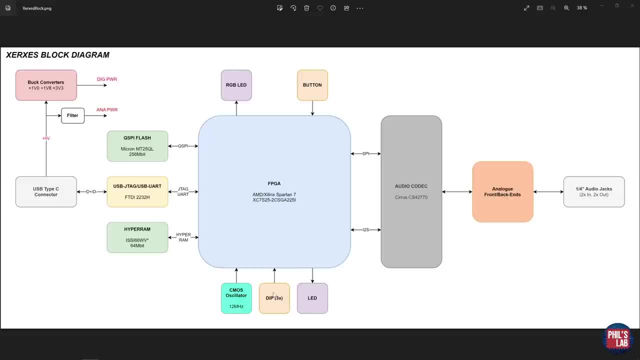 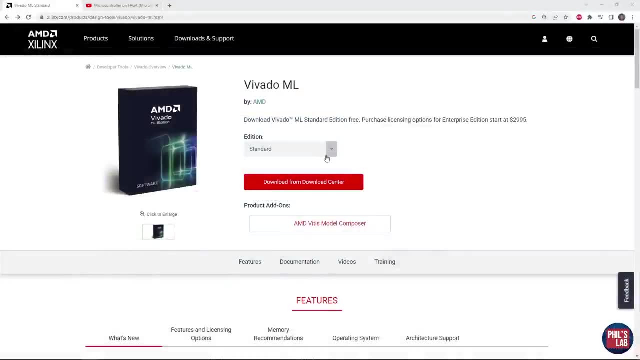 these DIP switches. A very, very simple example, but hopefully this will show you how to do it. you the flow of creating your own HDL and setting up your own project on custom hardware. I'd strongly suggest following along, and if you'd like to do so, I'll leave a link to this in the 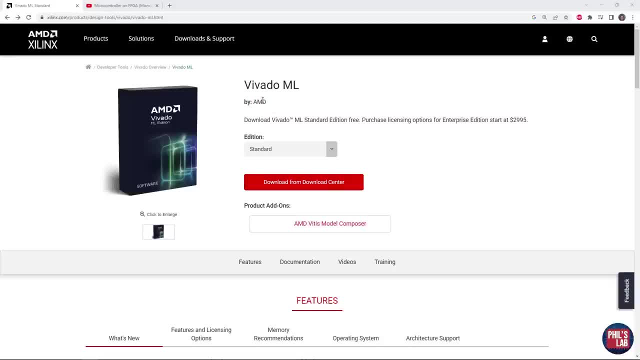 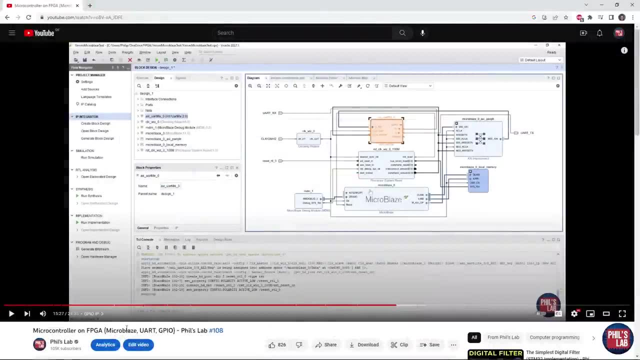 description below, but I'll be using AMD Xilinx Vivado tool, which is free of charge for these types of devices. On another note, if you'd like to see how to implement a soft core microcontroller on an FPGA, please watch the previous video, video number 108, on my channel. The first step is of 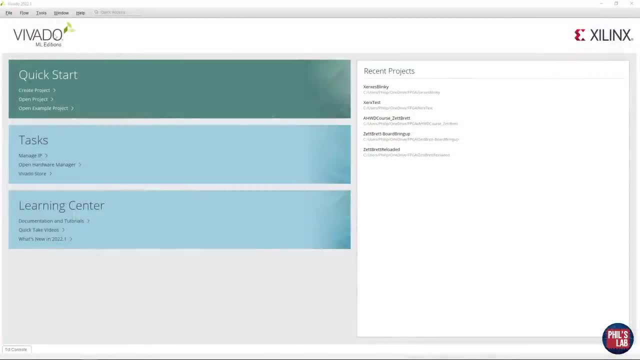 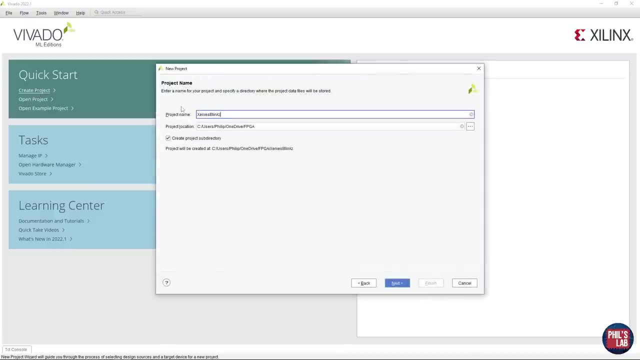 course, to launch our tool, Vivado, where we'll be doing all of our development in. Then we'd like to create a new project. simply click on create project. give it a project name. I'll just call this: Xerxy blinky demo. click next. We're not going to specify any sources at this. 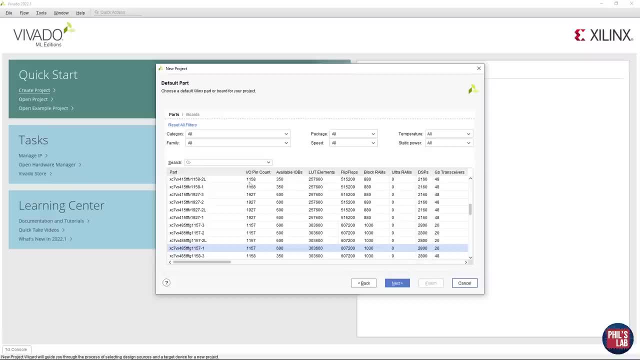 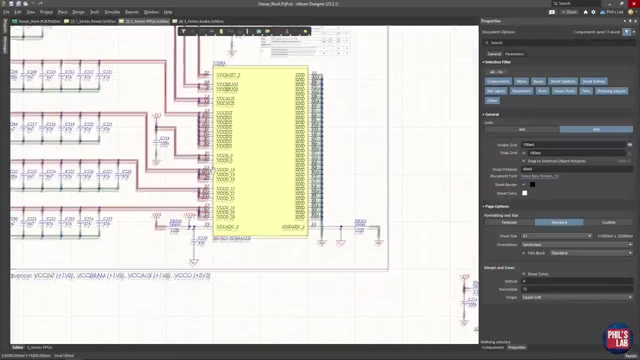 time, but we'll keep it as an RTL project. And now we need to choose our part. Remember, we're starting without any board definition files. we're just starting with our FPGA part. Going to the schematic and looking at the schematic symbol or one of the schematic symbols, we can see this is: 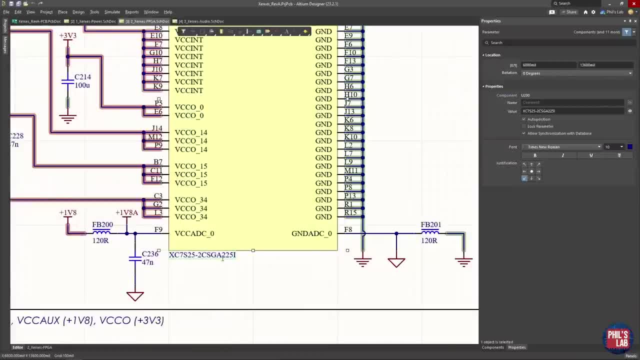 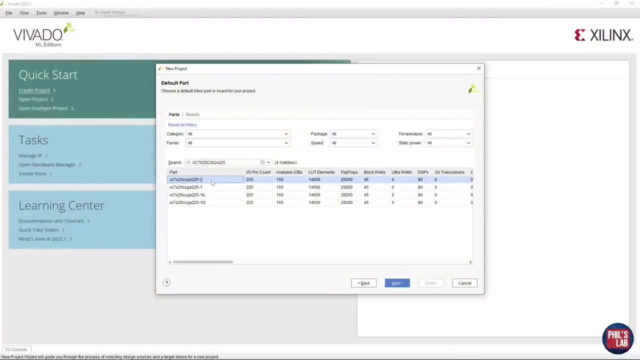 an XC7Z25 in a particular package- speed grade and temperature grade. So if I copy that over and type that in, we can see we have various different speed grade options and I'd like to choose speed grade two, which is the part I chose for this board. Select that and click next and 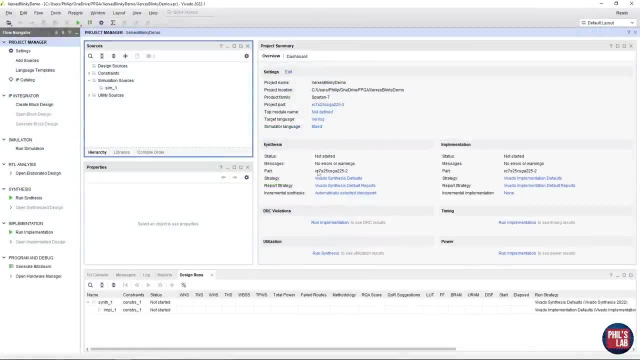 finish. Here we have a completely empty project which is centered around our part, the part we chose. The first thing we'd like to do is create the logic that will flash our LED. To do that, you can either write this in VHDL or Verilog. I'll just go with Verilog for now To create a module. 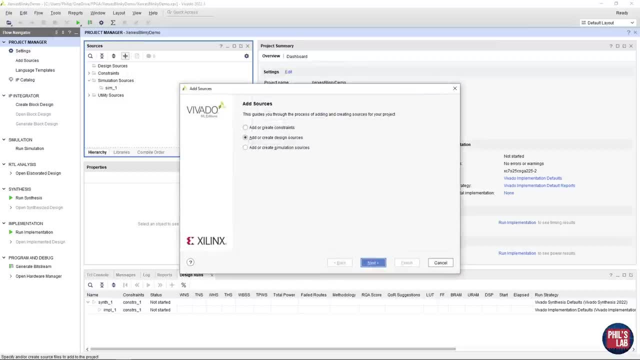 we simply go to the sources and click on plus and click on add or create design sources, then next, and then create file. This will be effectively our top file. this will implement the logic we need to link our dip switch and our clock input to an LED output. We'll just 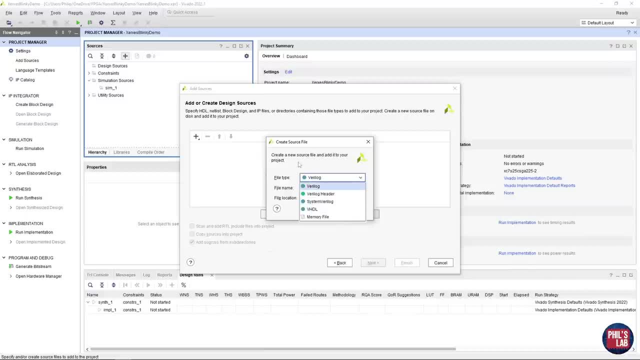 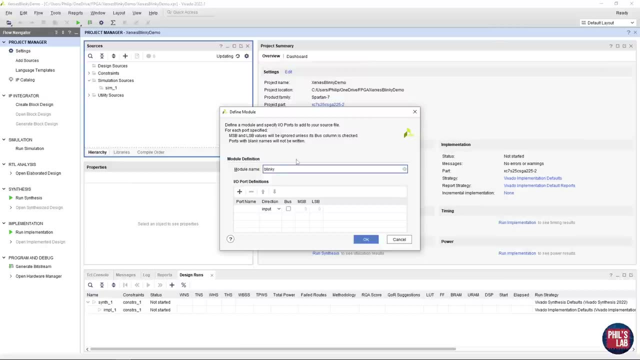 call this blinky, and okay, Of course you can choose a different HDL if you want. Then click finish. Keep in mind this video isn't an introduction to VHDL or Verilog or the like. there are many different tutorials on this on the internet and I'll leave a link to these in the 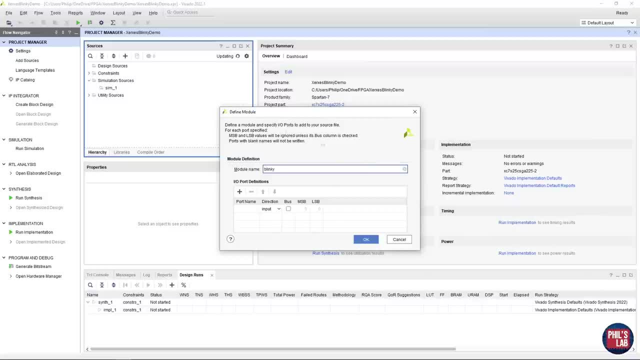 description below, But I'll show you the basics in this video. You can either ignore this define module or define in the description below. You can either ignore this define module or define in the description below. You can either ignore this define module or define. 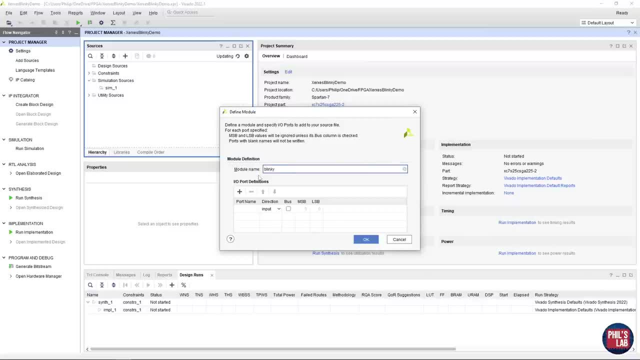 inputs and outputs to the module. Effectively, we're creating a block which we can then interlink with other blocks and these will have inputs and outputs and do some function in the middle. very simply speaking, We can define a port, For example: 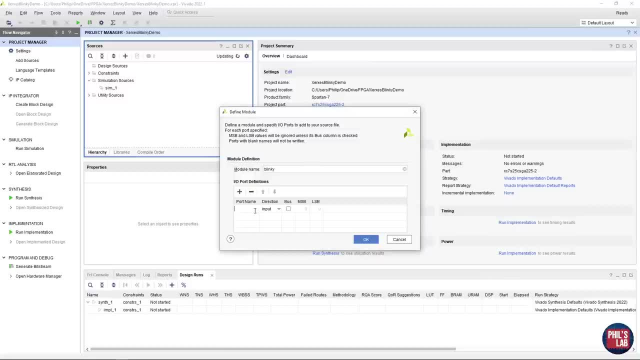 we're having a clock input- and let's just say this is a fairly arbitrary choice- but maybe a 10 megahertz clock input. So I'll denote the port name by clock 10, 10, indicating 10 megahertz Direction, is an input. We'd also like to control the frequency at which. 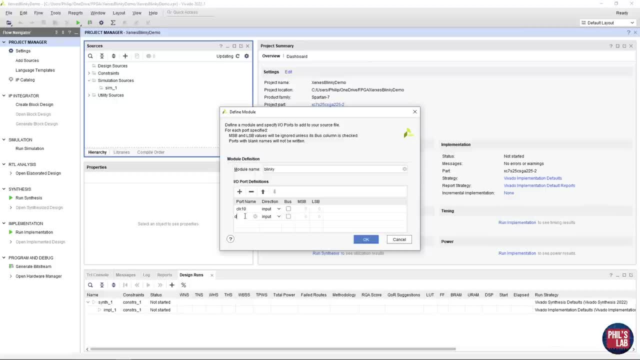 our LED is being toggled by one of the dip switches, So I'll just create another port name input and then input. So I'll just create another port name input and then input. So I'll just create another port name input and then input. So I'll just create another port name input and. 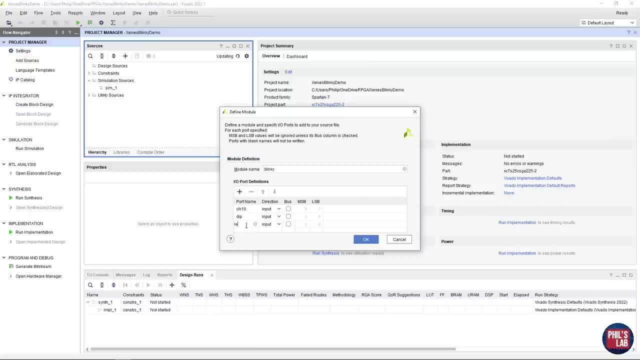 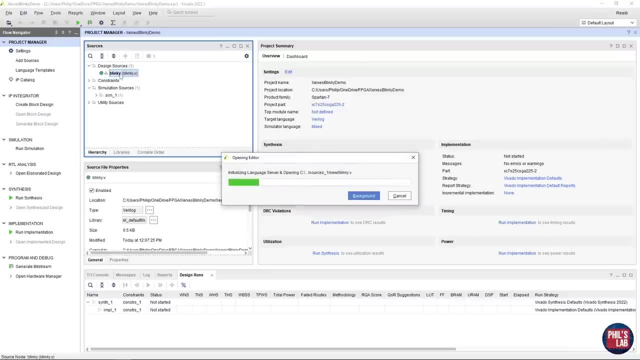 we of course want to toggle an output, which is our LED, So I'll just type in LED and set that to output, then click OK. Uvada now has created a module for us, Blinky, and set this as the top. 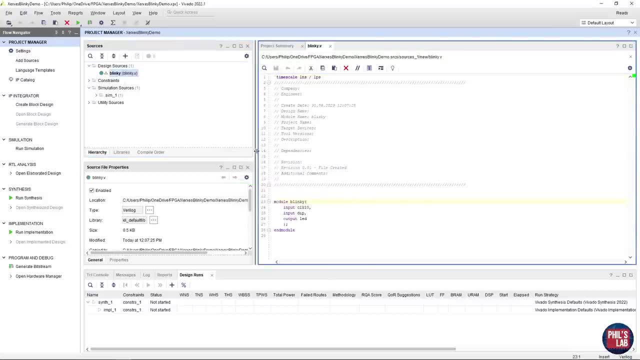 module. I can double click on this and this is what we see has been created by default for us. Let me just remove this at the top because it's not necessary and what we are now left with is a module definition. We have a module, the module name, what inputs we have. So we have a clock. 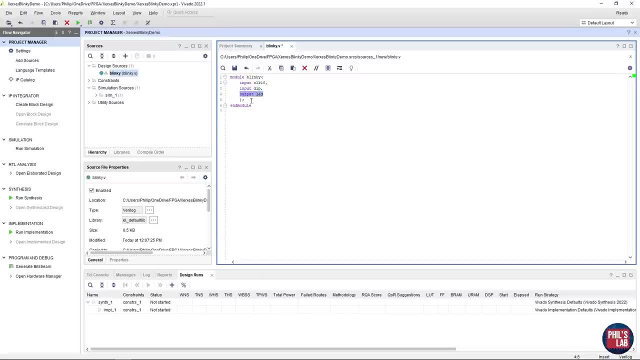 a 10 megahertz input, a dip switch input and an LED output Between the module and end module. we have to implement our logic. The question now becomes: how do we toggle an LED with a certain frequency, maybe a certain on and certain off time, given a certain input clock frequency? 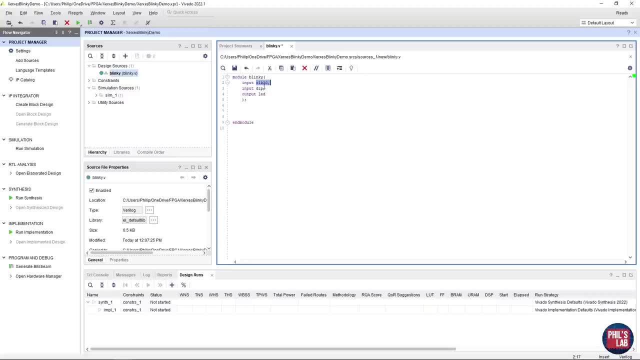 Our input clock frequency- arbitrarily in this case- is set to be 10 megahertz. If we were to flash the LED at 10 megahertz with our human eyes we would just see it constantly on LED because it's toggling far too fast. So we need to step down this 10 megahertz. 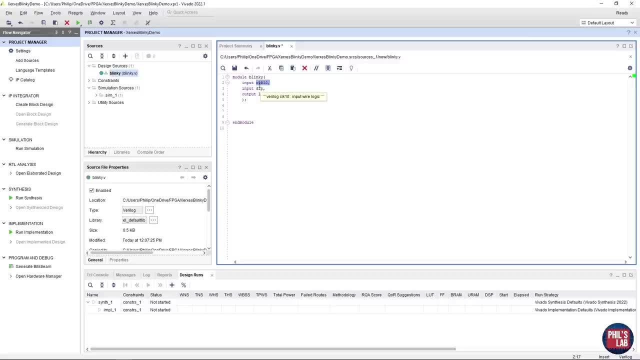 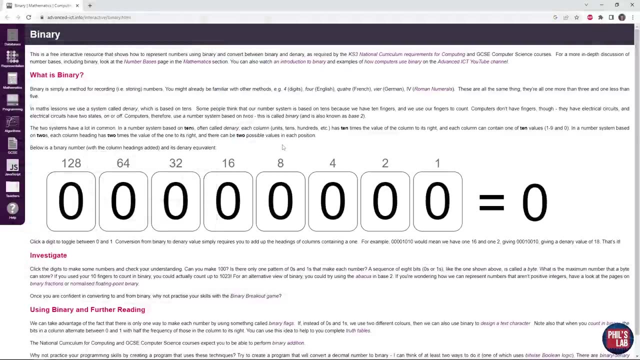 clock to maybe a one hertz or half a hertz signal, but how do we even do that? It turns out, of course, that there are several methods of doing this, and I'll show you a very simple and rather crude way of doing this. The way we're going to be doing this is by using a binary. 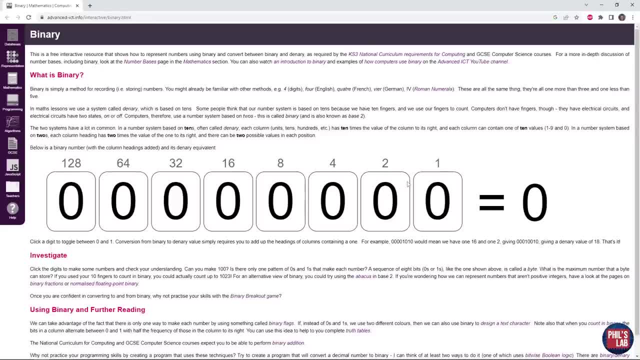 counter effectively a variable which we increment at every cycle of our 10 megahertz clock, So 10 million times per second. we'll be adding one to this counter. The counter will start at zero. The first 10 megahertz clock cycle will add a one, Then at the next clock cycle add another one and 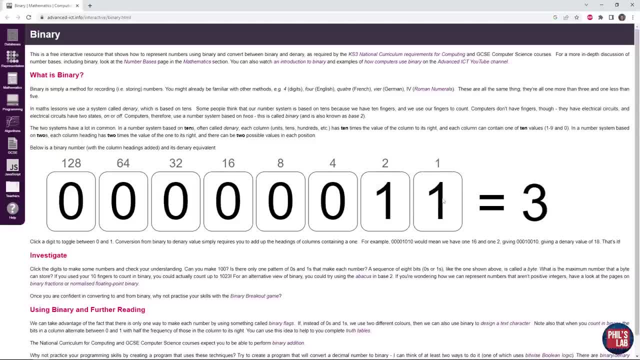 increment this to two. The next clock cycle, add one. increment this to three, then to four, to five, to six, to seven, and so on. If we look at the individual bits of this counter, we can see that, after a certain amount of time has passed, the individual bits, for example, bit which indicates: 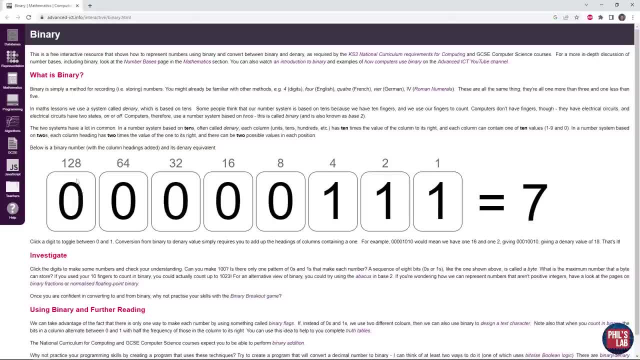 the 32nd position, 64th and 128th will change after some time has elapsed. So, for example, we could toggle the LED after the seventh bit has been set, and that will take 64 clock cycles. Or we can wait until the eighth bit has been set, and that will take 128 clock cycles, For example. 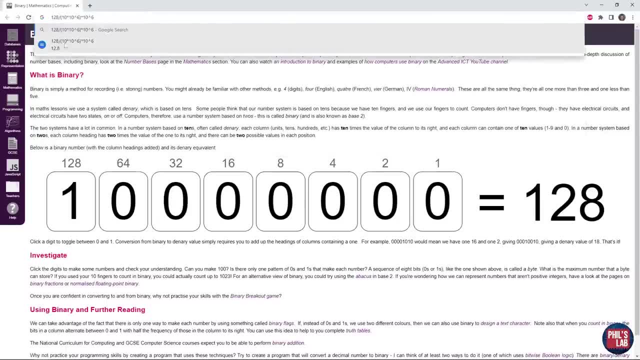 128 clock cycles at a frequent time. So, for example, if we look at the clock frequency of 10 megahertz, we'll take 12.8 microseconds. You can immediately see we need far more bits in our counter to create a longer delay. So for 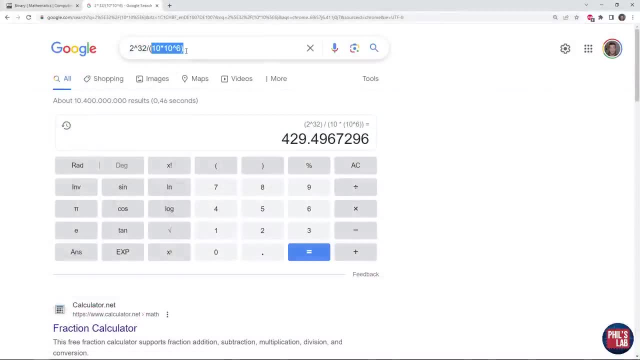 example, if we have a 32 bit counter, so 2 to the 32, divided by our clock frequency, which is 10 megahertz, we get a maximum period of 430 seconds If we use, for example, 20 bits of that counter. 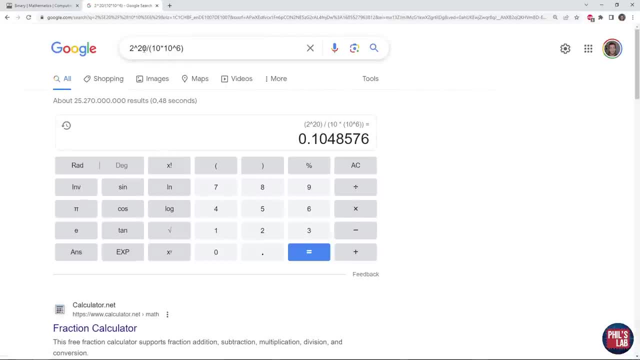 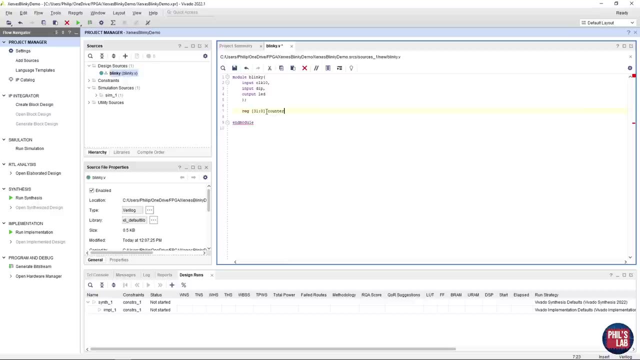 we get a period of 0.1 seconds and so on, And this is exactly how we're going to implement this Blinky, And this is a very, very simple way of doing it. The first thing I'd like to create is a counter which has 32 bits. We'll just call this counter. 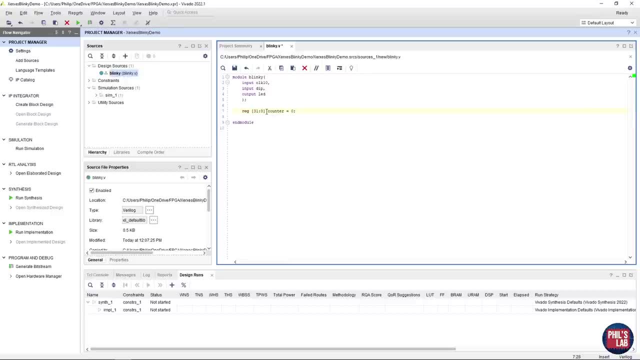 and set the initial value to zero. We could, of course, create a lower bit count counter, depending on what maximum lengths we want in terms of delays. We'll also then store the state of an LED as an internal register, which will then get fed or assigned to the output. 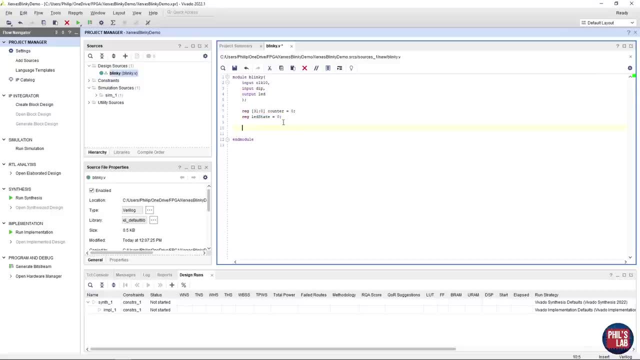 which is our LED output. This is an internal state. We can then simply assign the LED state to the output by using a Verilog assign statement. So the LED is simply set to the LED state, and that's what we're going to do. We'll just set it to the variable state, and then we can. 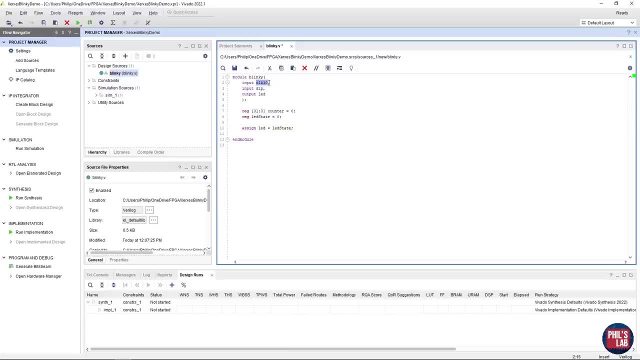 use the variable state to add an internal register. Now we want to increment the counter, this internal counter, every time the clock 10 input, our 10 megahertz clock input, fires. The way you do that in Verilog is do an always statement and always at the positive edge of. 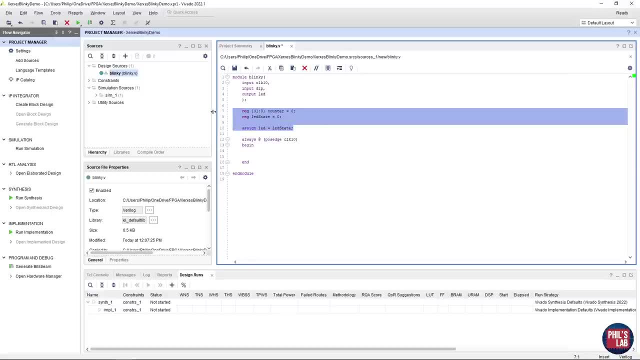 our input clock. we want to implement some logic within that always block, So the statements before effectively are set once we initialise our counter and our internal state and we make sure that our LED output is set to the internal state at all times. 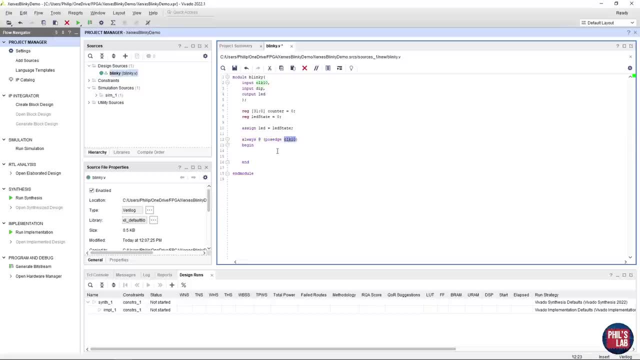 always at block the positive edge of our 10 megahertz clock input. So this block is effectively always fired or triggered every time we have a rising edge on that input clock. The first thing we want to do is increment our counter So our counter is assigned the value it had previously. 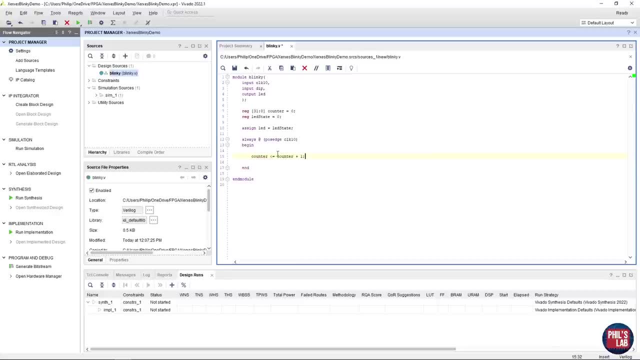 but we add one. The next thing you want to do- because now this counter is just free running- it'll increment at every clock cycle, so 10 million times per second, And once it overflows it'll return back to zero and then increment again continuously. However, this doesn't change. 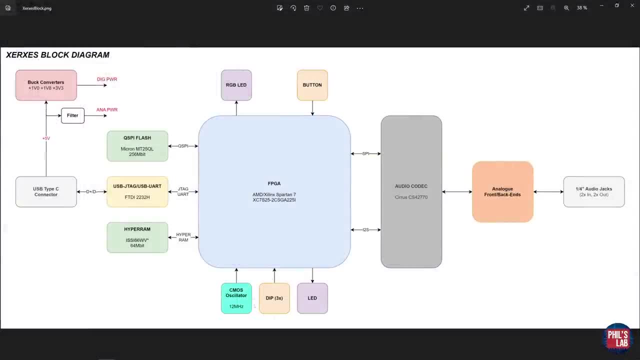 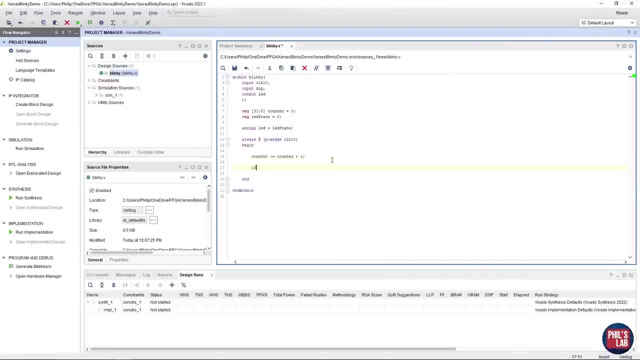 anything of the LED state. Remember, we said we want to have one of the dip switches mapped so we can change the on period or the frequency we are toggling our LED with. So, depending on if the dip switch is on or off, we want to have the LED have various on periods. Thinking back to our binary, 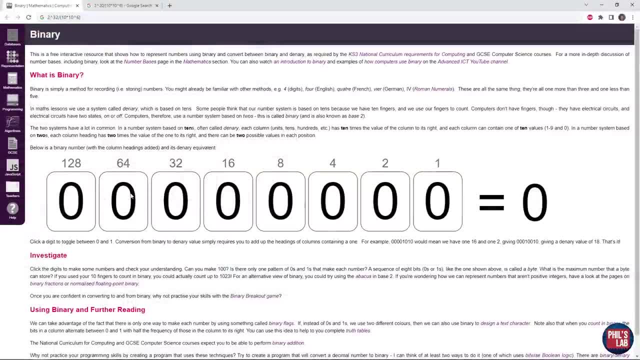 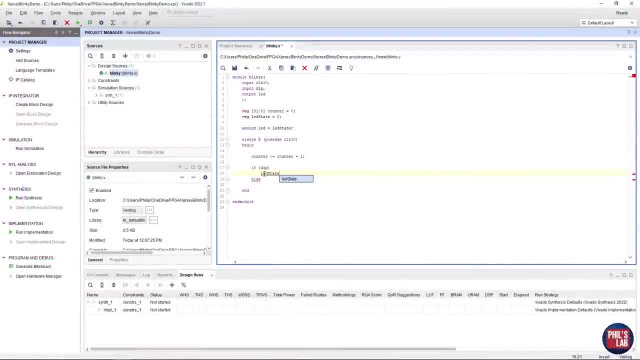 counter to then set the on state of the LED. all we can then do is choose one of the bits of our binary counter and assign that to the LED. So, for example, if the dip switch is high, we would like to have a higher frequency, so a shorter on period. If the dip switch is high, we would like to have 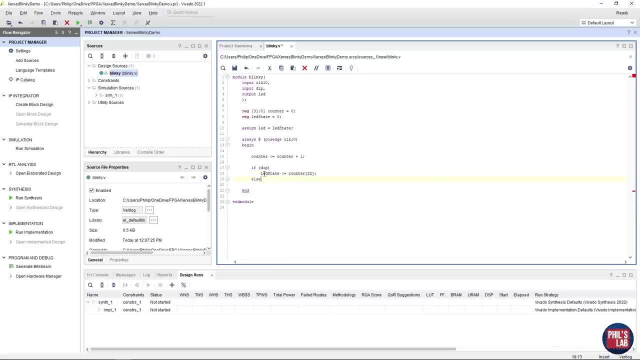 a shorter on period. So we'll just set that to, for example, the 22nd bit of the counter. If the dip switch is low, we'll simply set the LED to be the 23rd bit of the counter and therefore we have. 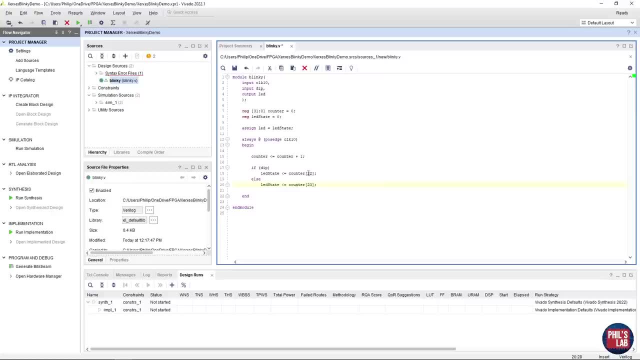 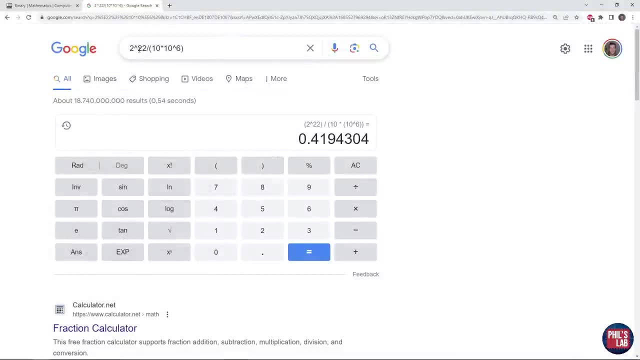 to wait longer for the LED to turn on and then to turn off. The question is: what on time and what off time do these bit positions indicate Approximately? if we're looking at the 22nd bit of our counter and toggling our LED based on that single bit, it's 2 to the 22 divided by 10. 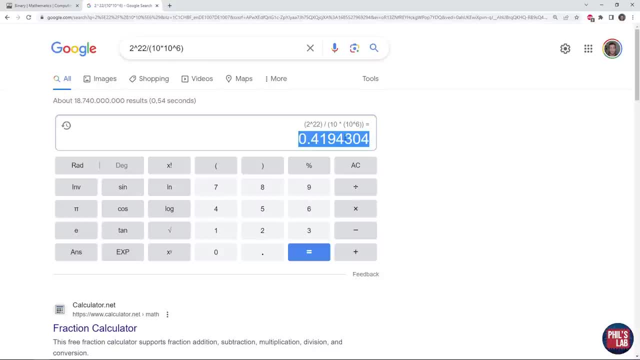 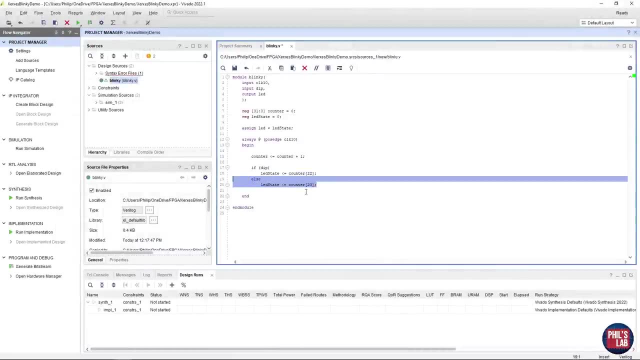 megahertz, which gives us an on and off period of about 0.42 seconds. And this was if the dip switch is high. If the dip switch is low, we move up one bit and, looking at the 23rd bit, and that simply is multiplying by two. So therefore we have double the on and off. 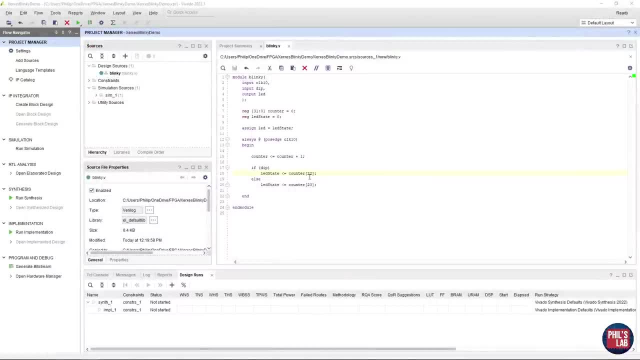 period, which is about 0.84 seconds. Remember, this is a very, very crude implementation. We're not looking for precise half a second or second values. We simply want to have a certain on period and a certain off period, depending on the state of the dip switch, And this is one of the easiest. 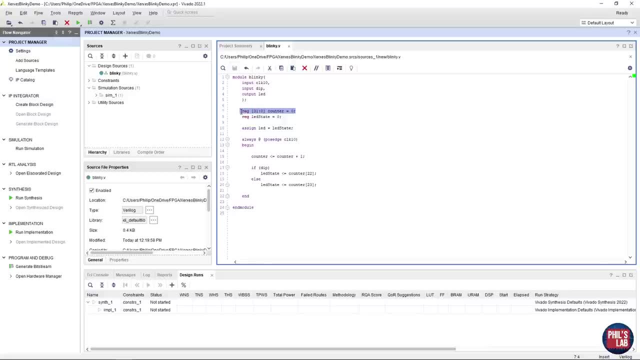 ways of how you can implement that. We simply have a binary counter. We look at individual bits of that counter, which is 0.84 seconds, And then we have a binary counter which is 0.84 seconds, And then we have a binary counter which is 0.84 seconds. And this is a very, very crude implementation. 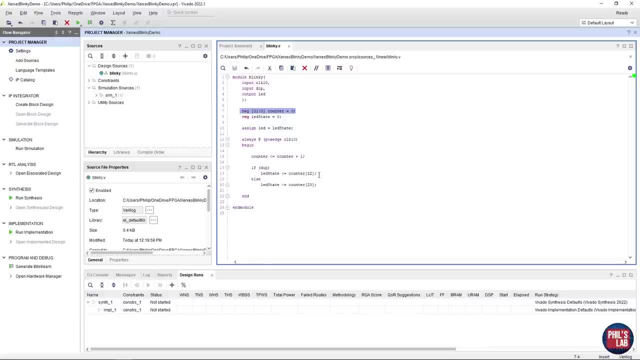 Then take longer to set, very simply speaking, and we set the LED state depending on those bits, either if the dip switch is set high or the dip switch is low. Every time we have a rising edge on the clock input at 10 megahertz. we simply increment that binary counter And that's all. 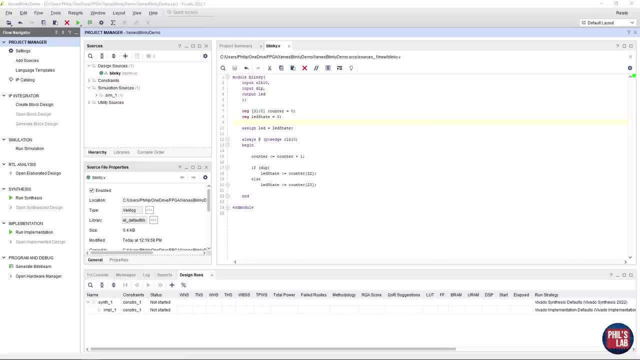 there is to this. We could straight away just implement this on our FPGA and see if this is working, but this is not typically the best thing to do. We would like to simulate our design first And, additionally, we don't have a 10 megahertz clock input, If you remember. back to the block. 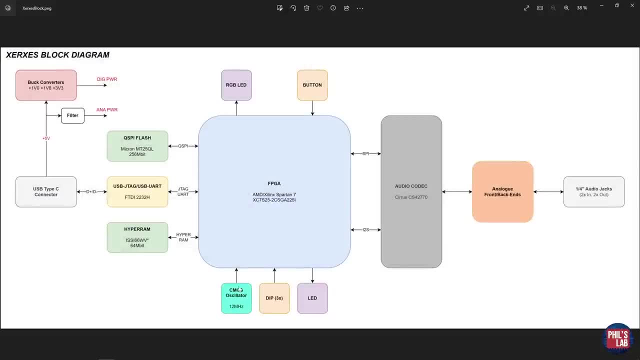 diagram. we have a 12 megahertz input, So how do we deal with that? We could either change, of course, this clock input to be 12 megahertz. That's fine as well, But I'd like to show you. 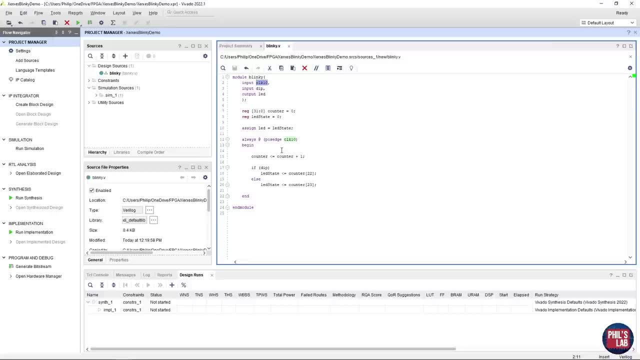 how to integrate that with a PLL or clocking wizard to adjust your input clock frequency- And that's why I've left this or change this to 10 megahertz input. In any case, before we get to that, we'd like to simulate our design and create what's known as a test bench for our module, The. 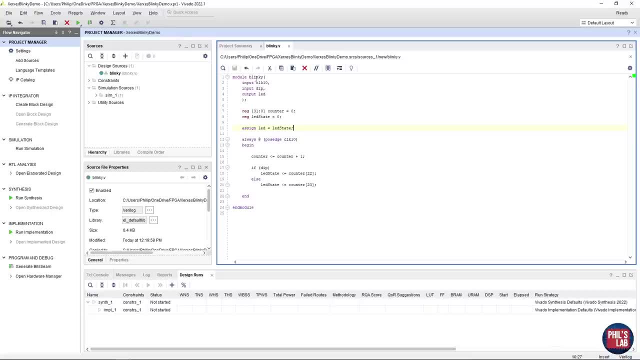 test bench in our simulation provides certain inputs and lets us look at the outputs for those inputs. So what we need to do is generate our own inputs. So what we need to do is generate our own clock and generate our input dip signal and then watch what the output does. in a simulation, The 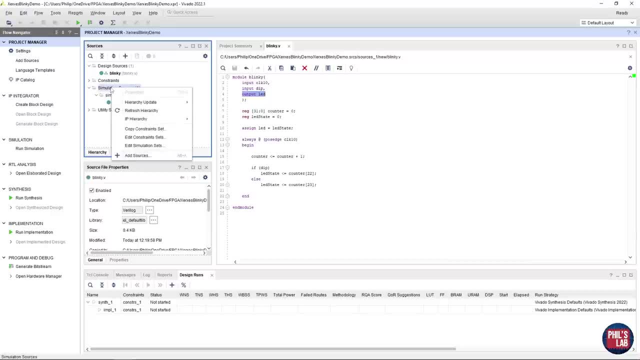 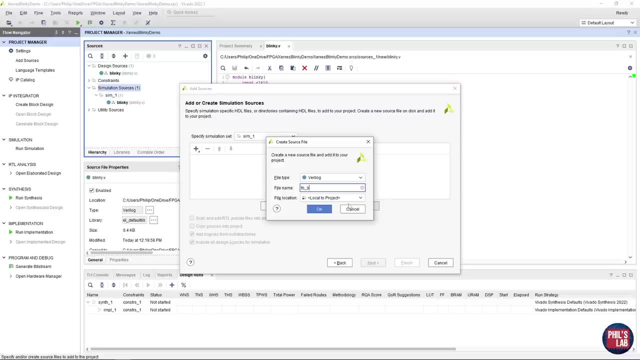 way we can do that on the left hand side, go to simulation sources, right click add sources and then add or create simulation sources. Then click next create file and I'll just call this TB. So test bench underscore blinky, and add that to the project. I'll just leave this all as default. 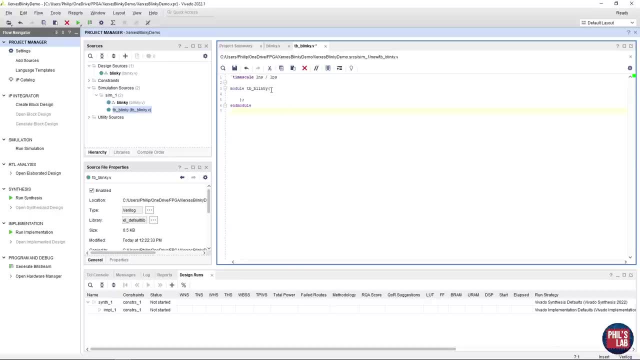 and click OK. We will then be greeted with this empty module including this timescale statement at the top. This timescale directive at the top is used for the simulation environment to find, for example, what our delay times are and what our precision is of the simulation environment. The fastest frequency we have in this design is: 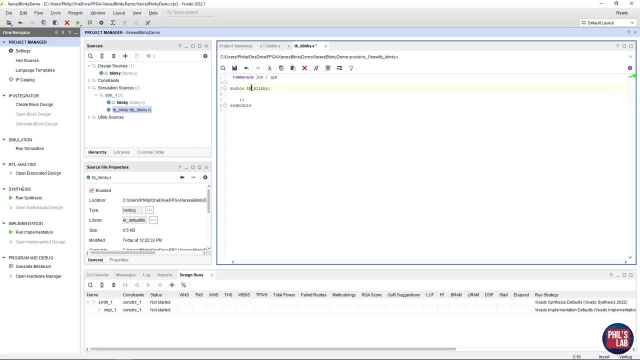 our clock 10 megahertz, which has a period of 100 nanoseconds. So we can either set the timescale to 10 nanoseconds. Since we want to toggle at a 50% duty cycle, we need to toggle our clock at 50. 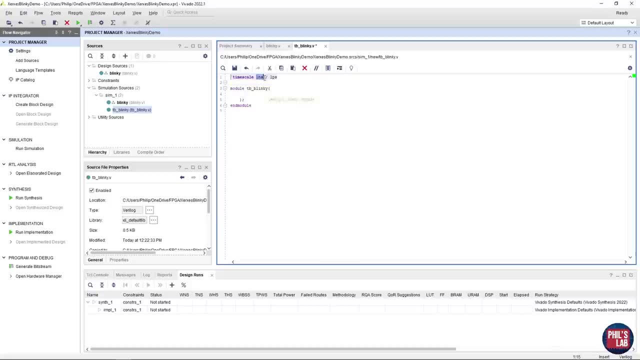 nanosecond intervals. Therefore, I've set my timescale to 10 nanoseconds, with a precision of 100 picoseconds. The test bench itself doesn't have any inputs or outputs, but we do need to define some registers. For example, we want to define the clock signal. We want to define the. 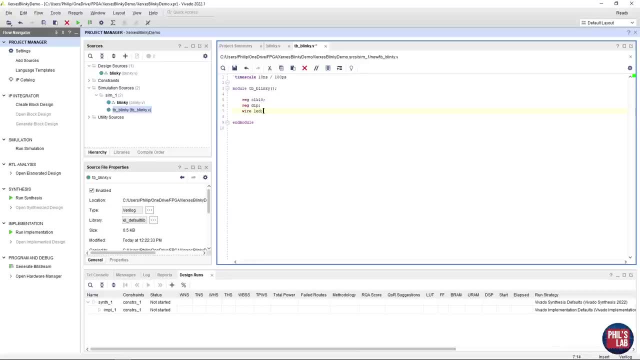 state of the dip switch and we want to check our output, which is our LED output wire. Then we want to instantiate our blinky module. We want to feed it- these clocks and dip switches- and read the output effectively at the LED. but we need to create our blinky module. The way we do that is: 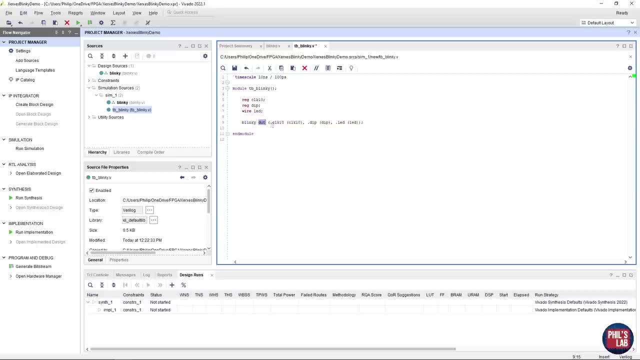 write the name of the module- We'll call it DUT- device under test and feed it, very simply speaking, the clock input, the dip, and set the wire output. Then we need to define what the clock and the dip switches actually are. Remember. 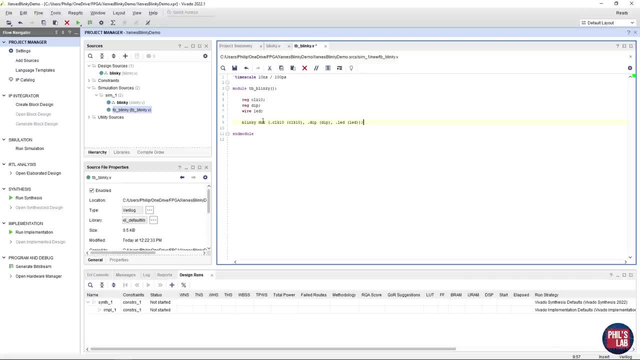 we want to feed these inputs to the device under test, which is our blinky module. To do this, we're going to do an initial statement as well as an always statement. The initial statement, as you can expect, is only run once when this module is initialized. 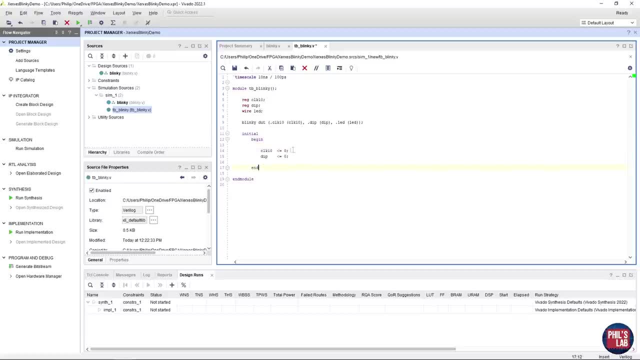 Something like this will suffice. We have an initial block with begin and end. We set the initial value of our clock signal to be zero and our dip switch for this test bench will simply be set to zero. Of course we could toggle that or change that, and we'll see that later. 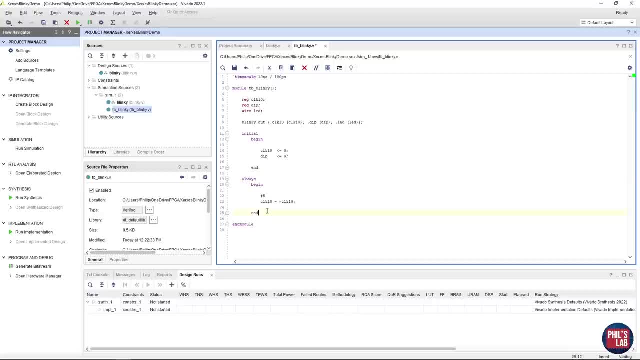 Next, we need to add in an always block, and this is effectively, as the name suggests, always fired. You can think of it as an infinite loop. very simply speaking, This hash 5 indicates how many time units we want to wait. If we have hash 5, this means we are. 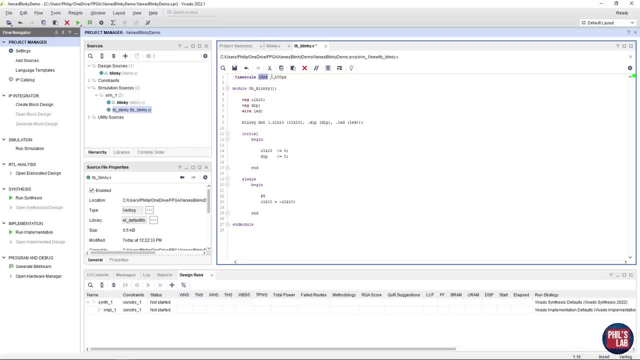 waiting for 5 time units. 5 time units are 5 times 10 nanoseconds which we defined up here. so we're waiting 50 nanoseconds before toggling the clock. We want to wait 50 nanoseconds because that's half our clock period. so we start with zero. we wait 50 nanoseconds, we toggle high. 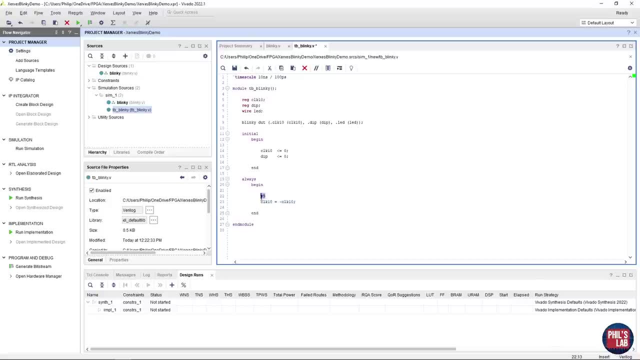 50 nanoseconds, toggle low and repeat that indefinitely. So we wait 5 time divisions, 50 nanoseconds. we set the clock is not equal to the current clock state. So since we started with a clock state of zero, the first time we encounter this we'll toggle to one, then wait 50 nanoseconds. 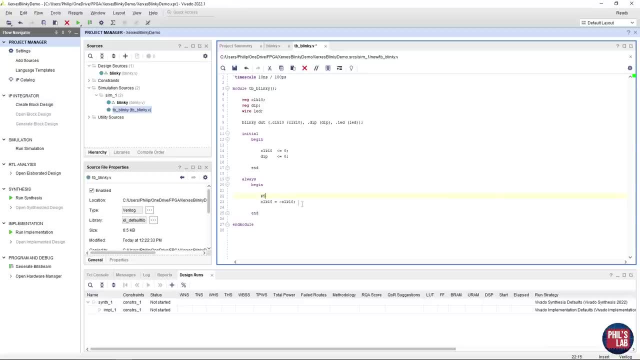 toggle to zero, wait 50 nanoseconds, toggle to one and so forth, And this is how we can very simply generate our clock signal, Now that we've written our Blinky module, as well as the test bench for this Blinky module, where we're simply setting the value of the dip switch and then 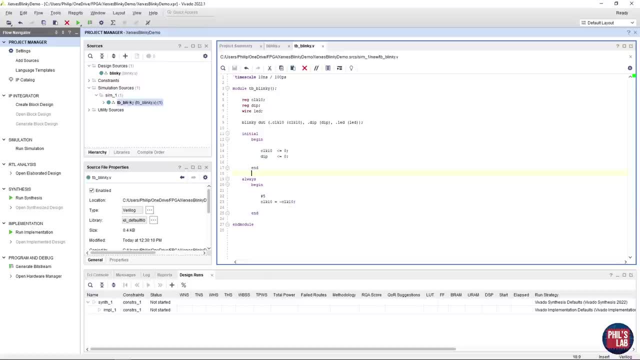 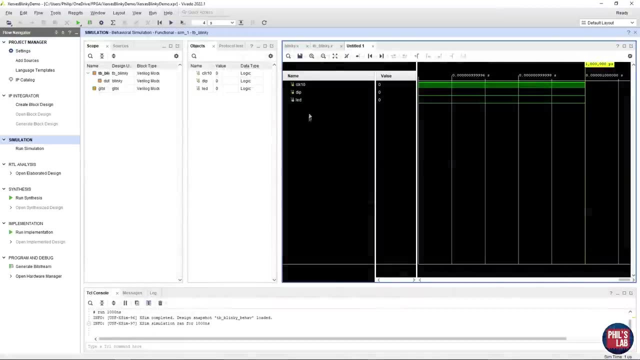 our clock signal at 10 megahertz. we now want to run the simulation. What we have to do on the left-hand side is then simply click on the run simulation, run behavioral simulation and our simulator opens up. We can see that we have our clock signal, which is visible. 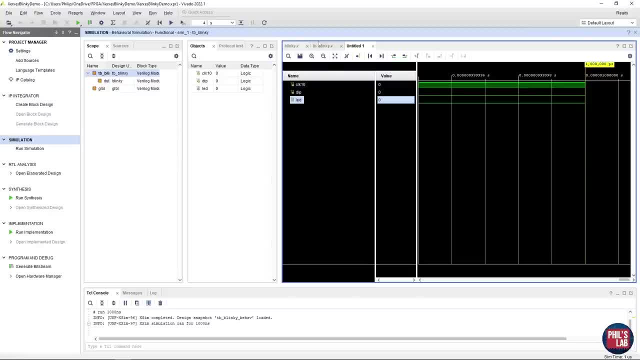 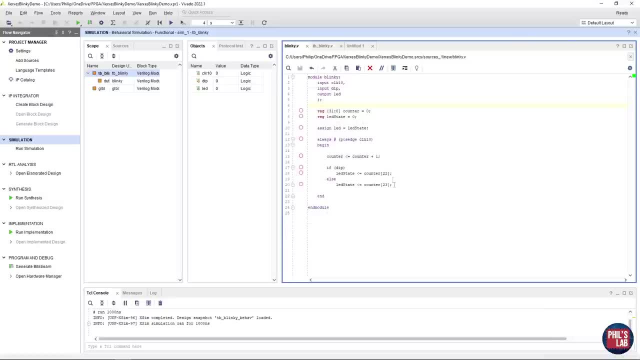 the value of our dip switch as well as the LED output, and this is based on the test bench and, of course, the underlying Blinky module. We had defined that our dip switch should initially just be low, meaning that we have the longer on state and longer off state for the LED. 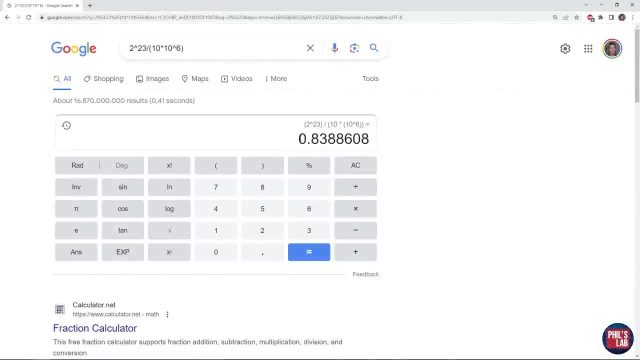 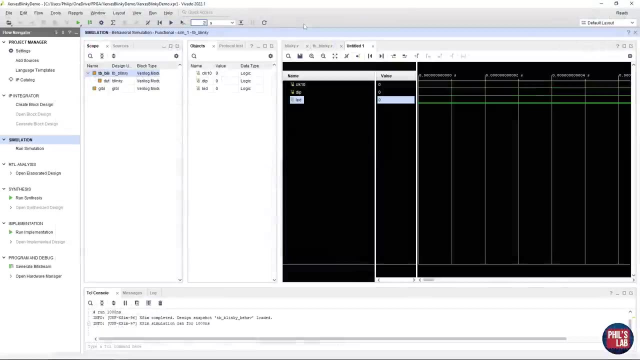 where we're looking at the 23rd bit of our counter. If you remember back, this should mean we have an on and off period of about 0.84 seconds for the LED, So let's see if the simulation reflects that. At the top I can enter how long I would. 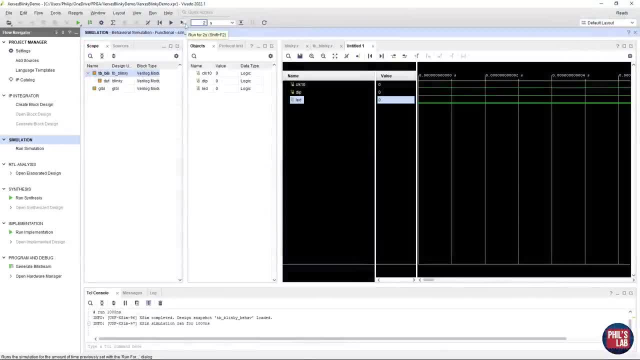 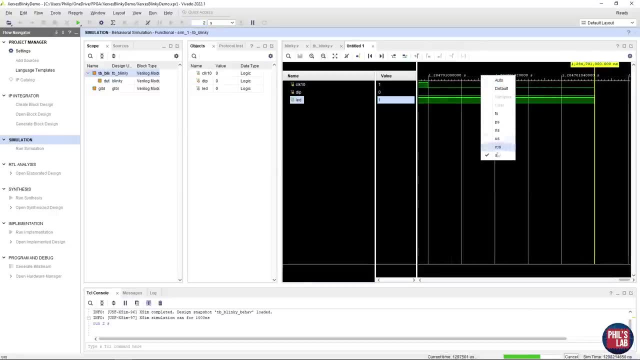 like to run the simulation, for I'll just run this for two seconds and then click run for two seconds. I can zoom out using the plus and minus in these magnifying glasses. If I right click on the top I can change my units of my time interval. I'm on seconds right now and just wait for the. 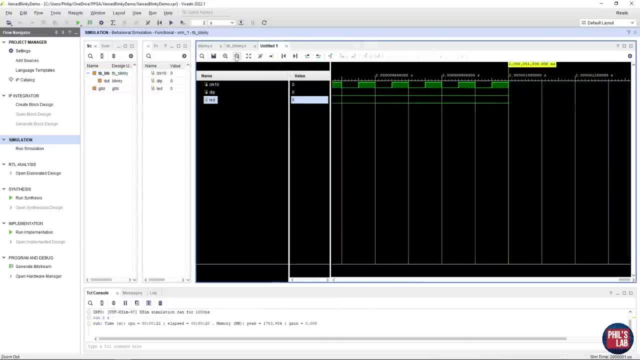 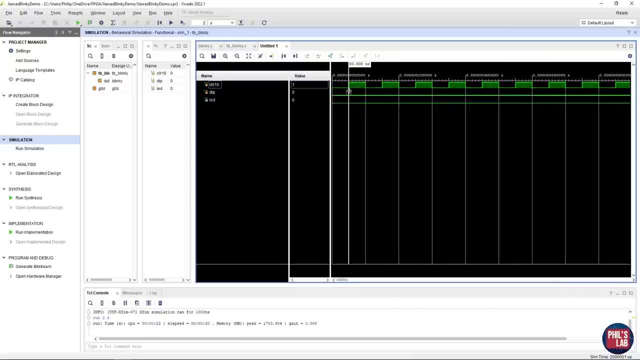 simulation to run. With the simulation finished, let's just zoom out a tiny bit and scroll back to the top. We can see our clock starts at zero, which is what we defined. After 50 nanoseconds goes high, after another 50 nanoseconds goes low, and therefore we have a clock period of 100. 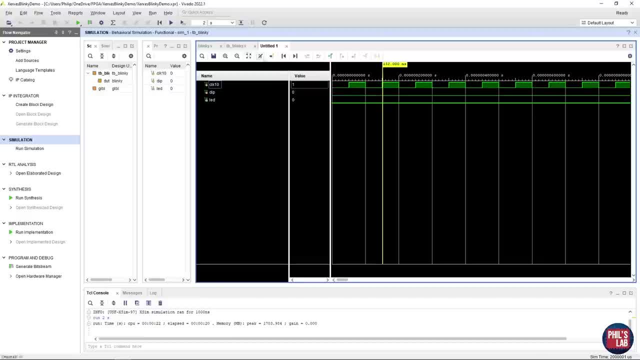 nanoseconds, which is 10 megahertz, and exactly what we specified in our test bench module. through this, always block Because the dip switch is low, as we can also see here, a logic zero. we should expect our LED to then turn on at intervals of 0.84 seconds. 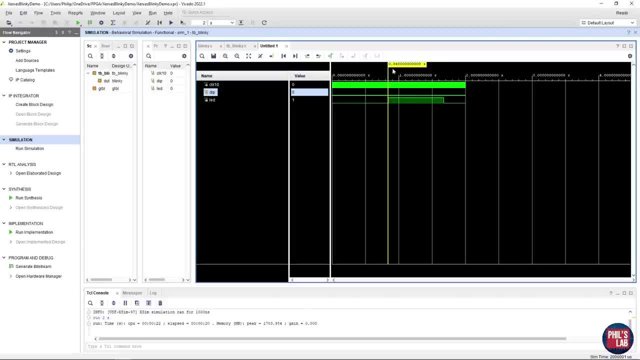 That's pretty much exactly what we get. So this is approximately going into 0.84 seconds. This is when our LED jumps to a high, and adding on 0.84 seconds of that, at about 1.68 seconds the LED. 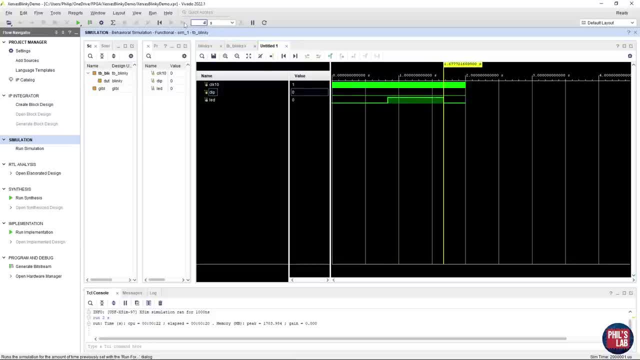 drops back down to zero. We could of course extend our simulation time run for another four seconds, and then we should expect our LED behavior to go on and off always at these fixed intervals and fixed periods, as we specified with our binary counter and our dip switch setting. And this is 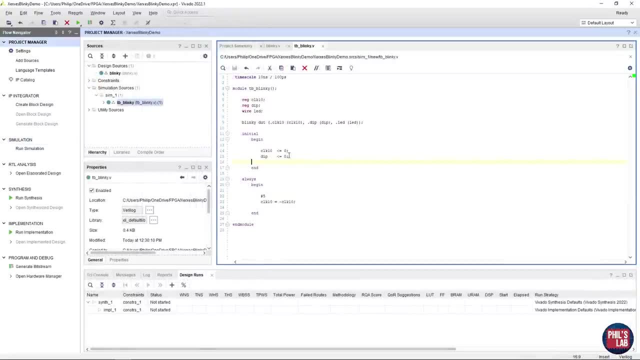 exactly what you can see here. So I stopped the simulation and now adjust our dip switch to be a logic one, meaning if the dip switch is a logic one, then the dip switch is a logic one. We now have half the period because we're only looking at the 22nd bit of our binary counter. 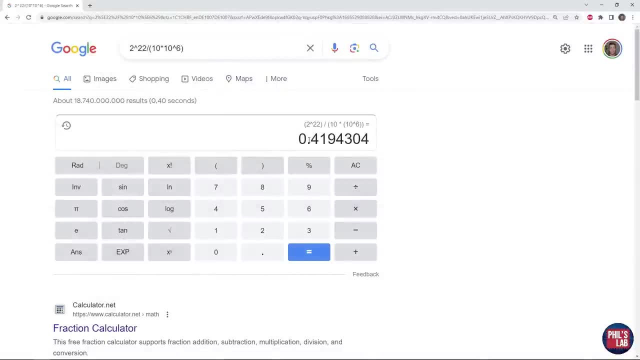 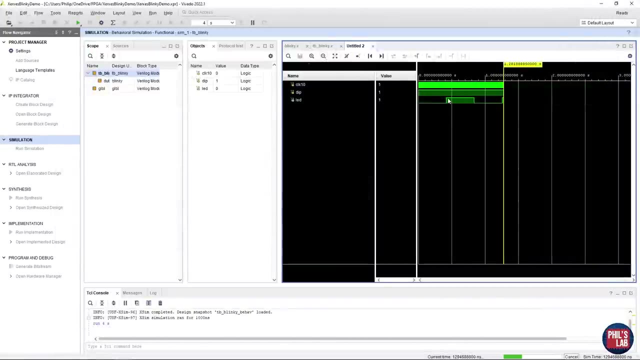 Rerunning the simulation. we expect a period of 0.42 seconds approximately. You can see the dip switch is now at one. If I zoom out further while it's running, we can see. now the period is shorter: half the on and half the off period of the previous setting. 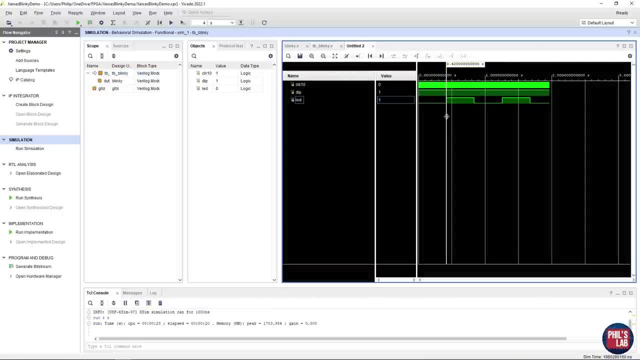 I'll just pause the simulation. So we get our initial on transition at about 0.42 seconds and at 0.84 seconds approximately we have our high to low transition, And every 0.42 seconds we have our transitions, as we expect from our Blinky logic. So this is great And this is what 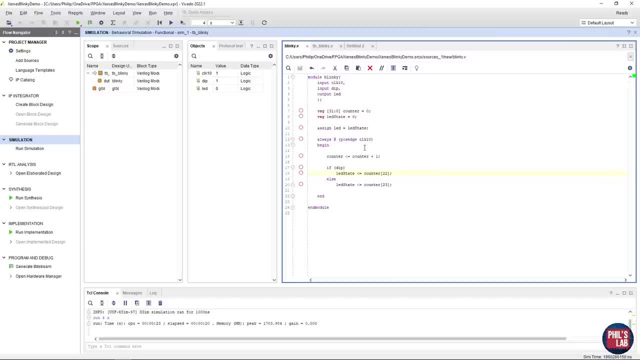 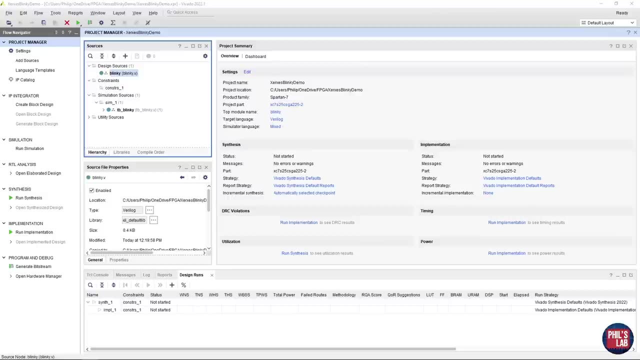 you should always do is do a simulation before you implement this on the FPGA. We'd like to move over to implementing this design on the FPGA and see if this works in the real world, so to speak, after we've verified it with the simulation. Remember, I said that the board is 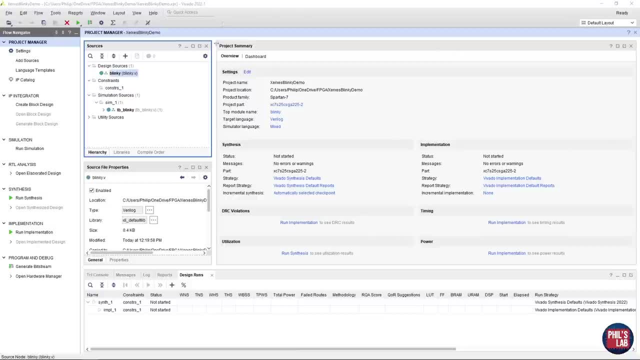 actually fed by 12 megahertz CMOS oscillator, but our Blinky module is expecting a 10 megahertz clock input. The reason I did this is because I'd like to show you how we can add in blocks and IP blocks and combine these IP blocks with our own HDL. So on the left hand side. 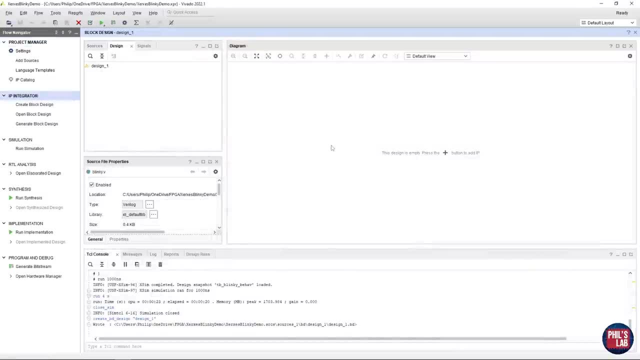 click on create block design. We'll just keep the default name for now. And then we'd like to add in our Blinky module. The way you can do that is right click, add module and then Blinky. And here we go. We can see we have our two inputs, which is our 10 megahertz clock input, our dip. 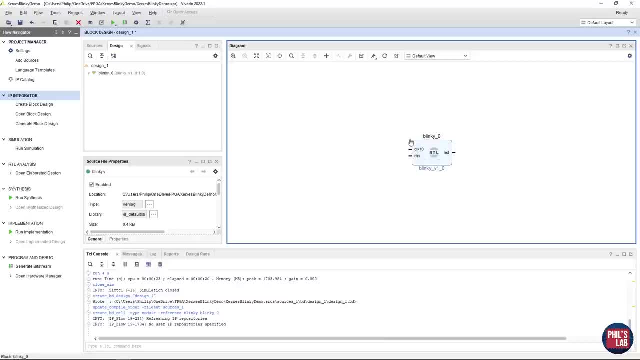 switch input and an LED output, And this is based on the definitions we did in the Verilog module. What we now need to do is, of course, create ports that then map to our real world design. So, looking at the schematic in the real world, for example, the LED driver is mapped to pin A2,. 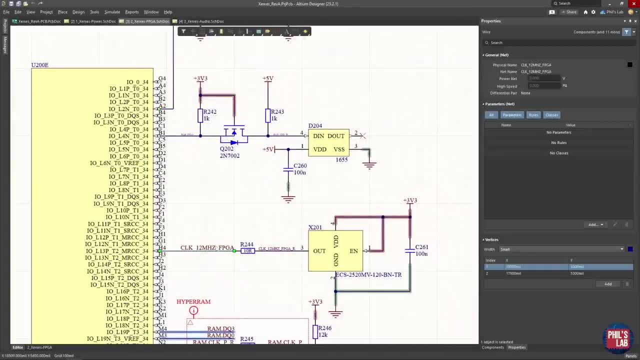 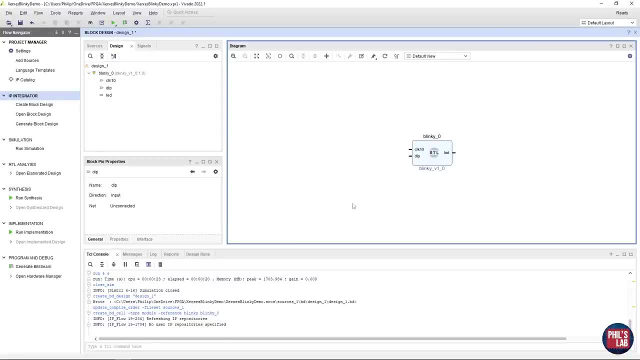 which we would define as a port, or my clock input, my 12 megahertz clock input is mapped to pin H4, and so on. We need to somehow add this in, first of all as ports, and then mapping those ports to constraints on the board itself, And let me show you how to do that. So, for example, 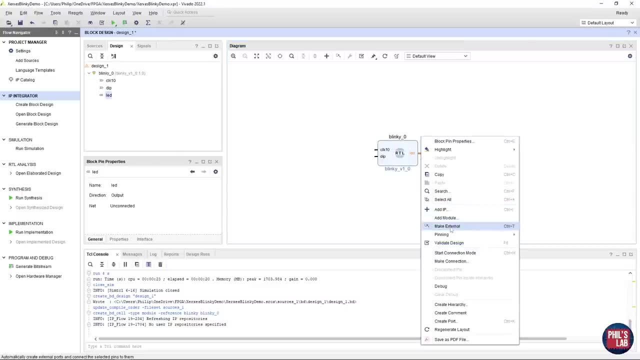 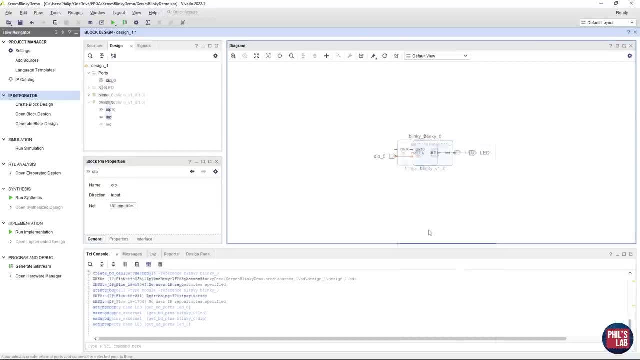 the LED. we can right click on that pin and click on make external. This will add this external port. I'll just rename this to capital LED. We can do the same thing for the dip switch: right click, make external and change its name to capital DIP. But now we have the clock, Remember. 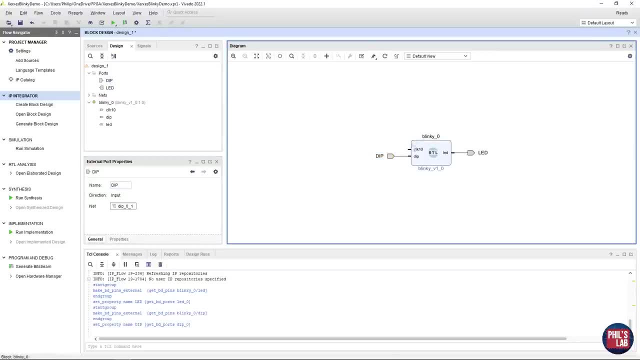 the board clock is actually a 12 megahertz oscillator. How do we get this to be now a 10 megahertz input that feeds our blinking module? Well, this is where I'd like to show you how we can combine our own HDL or RTL modules with pre-made IP blocks. So go to the top, click plus. 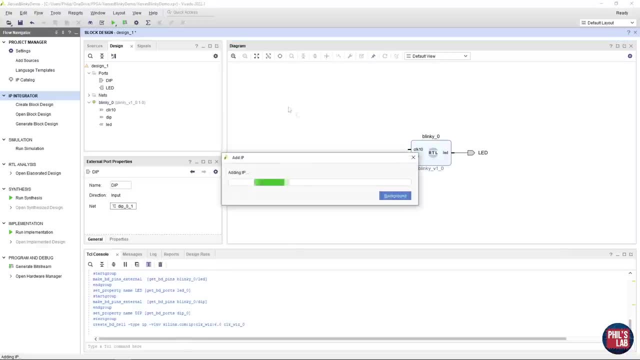 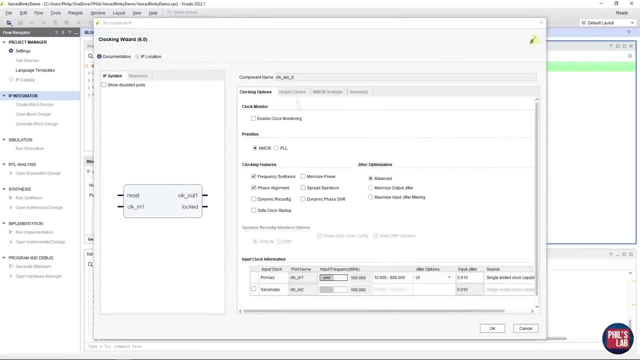 add IP and look for clocking wizard. Double click on that and that adds in a clocking wizard. If I double click on the clocking wizard, we can see that this takes in more clocks and on the other side we can output different clocks. So you can think of this very. 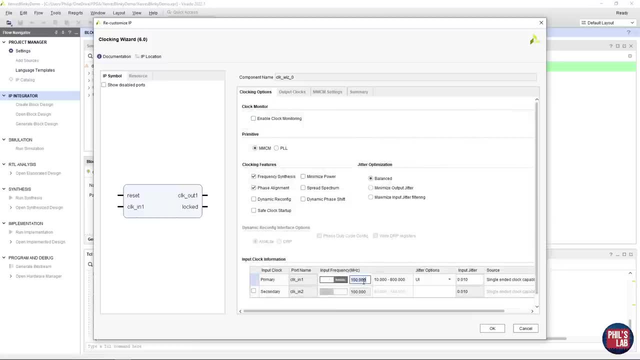 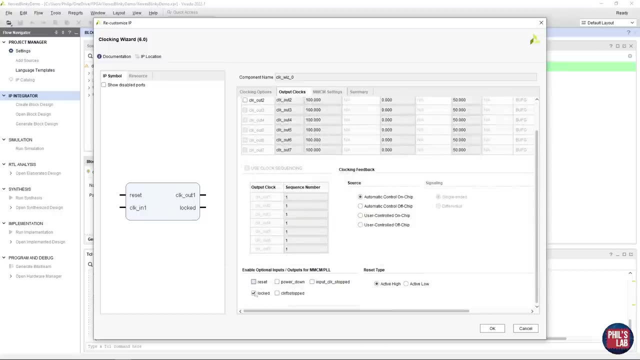 basically as somewhat, for example, a PLL, So we can set our input clock to be 12 megahertz on our output clock to be 10 megahertz. I'll just turn off these optional inputs and outputs for the reset and locked signal and click OK. So therefore this clocking wizard can take our 12 megahertz. 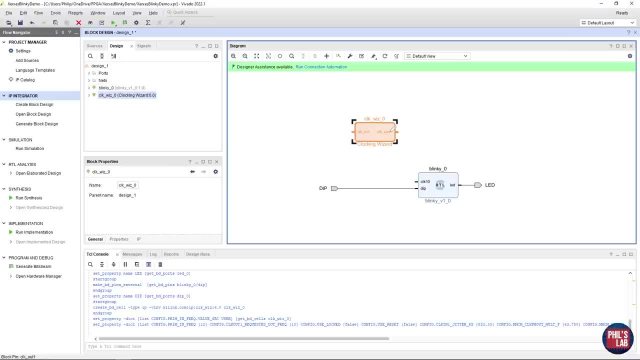 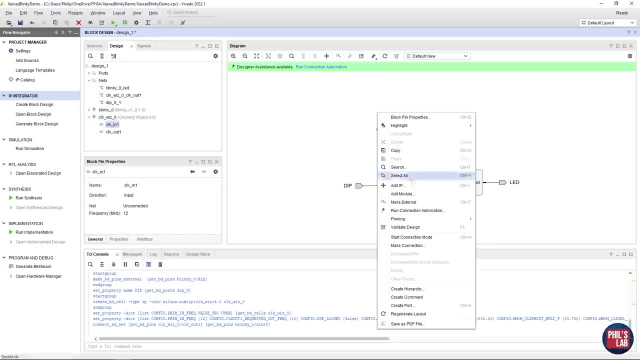 crystal oscillator input coming from the board and then reconfiguring that, very simply speaking, to be a 10 megahertz clock output, Then I can simply wire that up by dragging and making the clock in an external port, as we did before, and I'll simply call that. 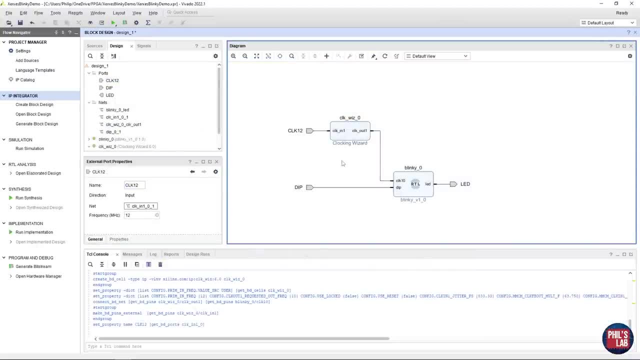 clock 12.. And this is how simply we can combine our own modules with pre-made IP blocks and then define the external ports. We've defined the external ports, but we actually haven't mapped these ports yet to physical pins on the device, as we saw just now on the schematic. The way I 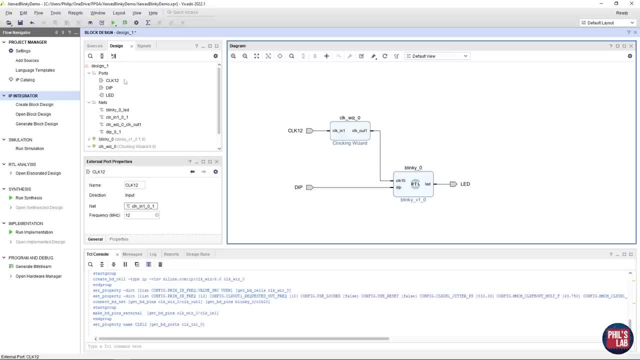 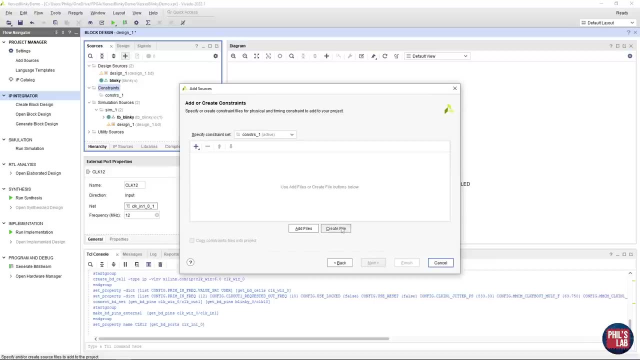 typically do that and there's many different ways of doing this- is going via a constraints file. So you're going to sources, click on the plus, add sources, and then add or create constraints And we'll create a constraints file. I'll just call this Xerxes, which is the name of the board. 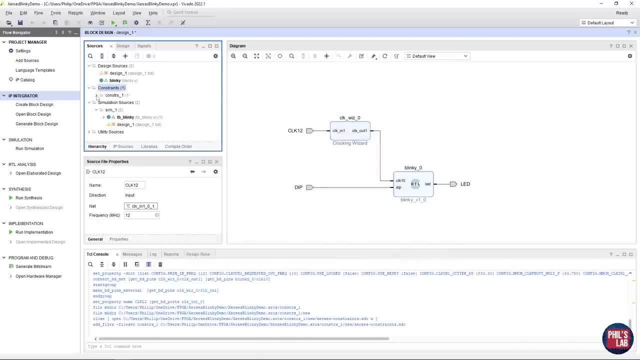 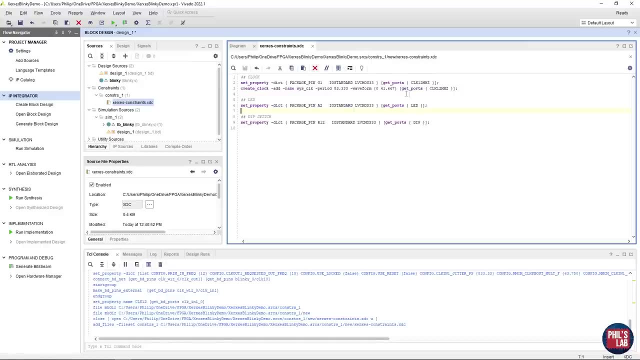 dash constraints, click OK and finish. Now in the constraints folder, in the sources block, you can see we have an XDC file which defines our constraints. I've copied in some constraints I previously had written And, for example, looking at the LED constraint, all we're doing is using 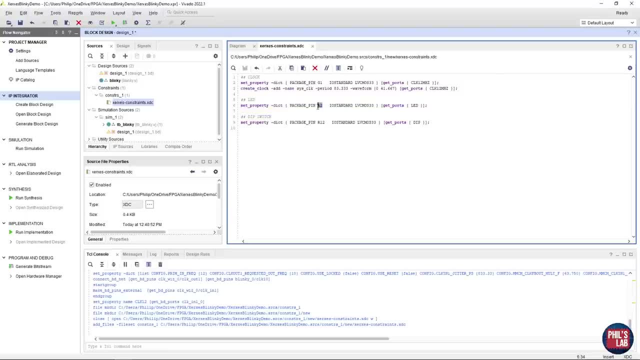 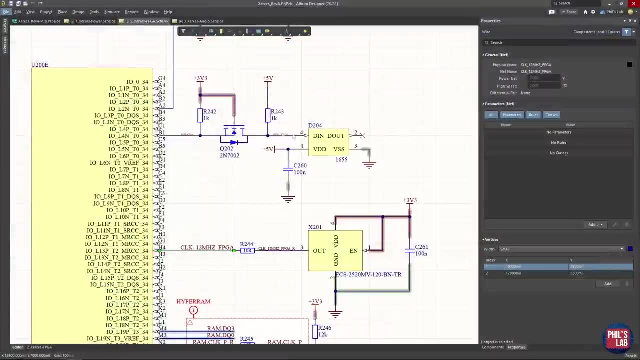 the set property command, telling our tool what package pin we're using- A2, what the voltage level standard is, which is a CMOS 3.3 volts, and assigning the port name LED. From the schematic that's simply pin A2 on the package pin. This is the LED driver for our run LED. Similarly, 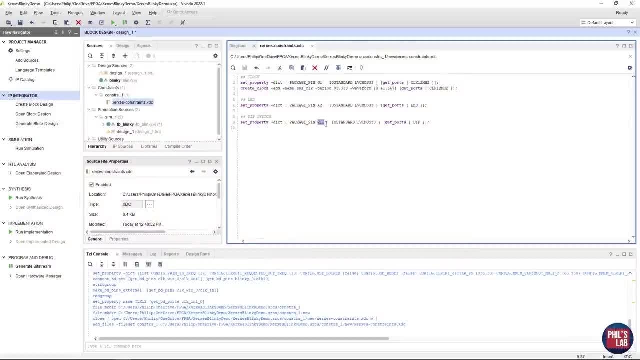 for a dip switch. I would run the same command. This time, our dip switch will be connected to pin R12.. Voltage level is 3.3 volts, which is defined in our schematic as well. That's what the bank is running off And we're running, and we're calling this port dip For the clock. 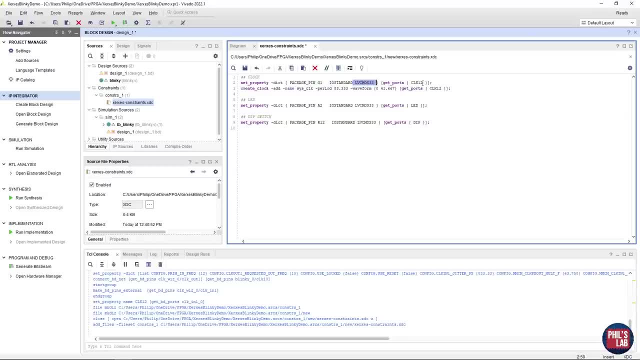 it's quite similar as well. We're defining the package pin, the standard, and calling the port clock 12.. But then we also have to define the clock period as well as the duty cycle, as in period for 12 megahertz clock is 83.3 recurring nanoseconds And our waveform is a 50% duty cycle. 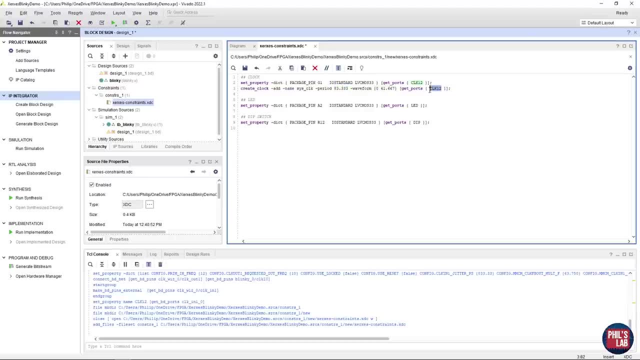 so it's zero to half the clock period And I'm assigning that to my port. You can see also the name of these ports. so clock 12, LED and dip is consistent with our block design we created here. So clock 12, dip and LED will then automatically get mapped to these constraints we defined here. 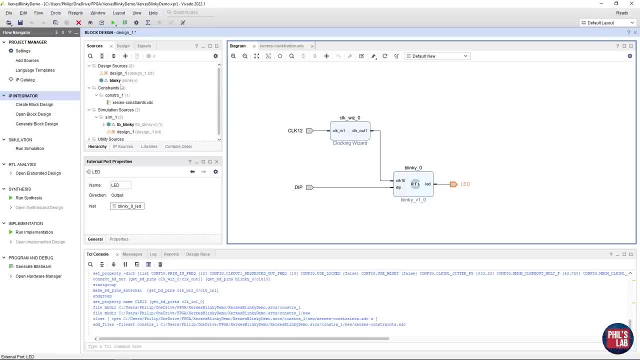 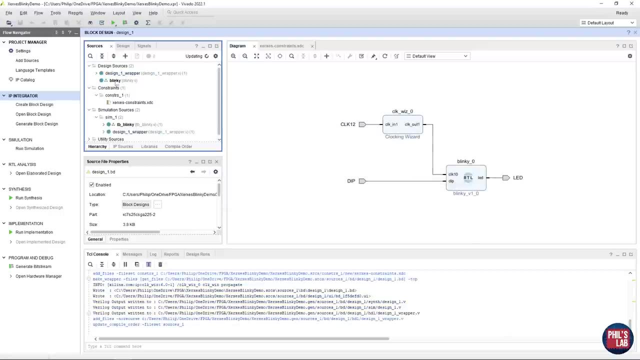 Once you're happy with that, we have to create an HDL wrapper for this block design. So right click HDL wrapper, click OK. What we can now see is that we've created this wrapper. Nicely enough, Vivado has automatically made our block design, which has now been wrapped in an HDL wrapper. 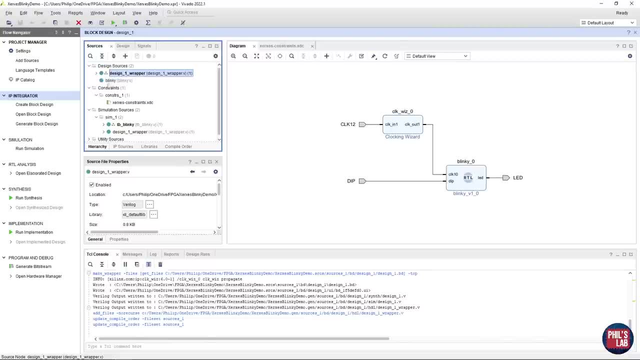 our top module. If this for some reason isn't the case- and, for example, Blinky might still be bold- simply right click and click on Set as Top. Once we've done that, all we have to do is run the. 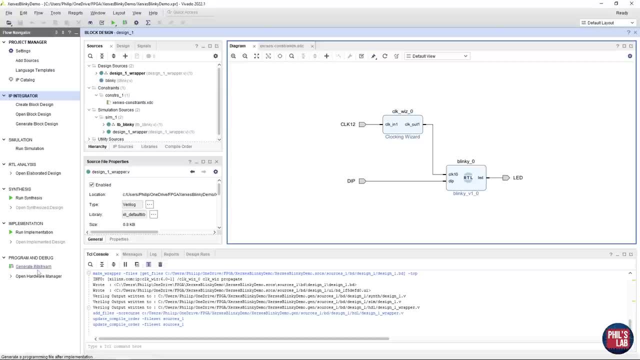 synthesis and run the implementation and then generate the bitstream. I won't be going to detail what synthesis and implementation are in this video, but if we click on Generate Bitstream, it'll run synthesis and implementation directly. So that's what we're going to do. 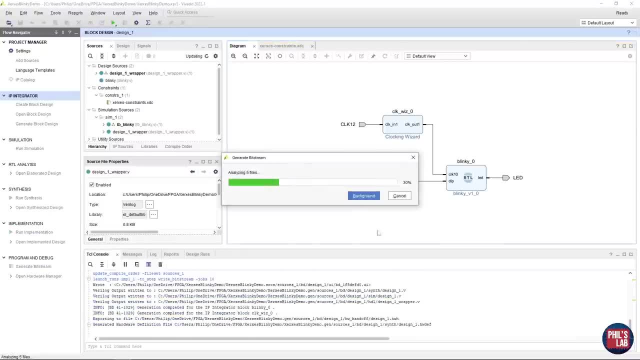 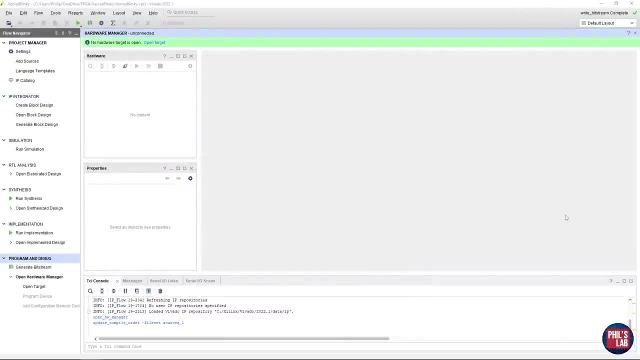 So that's what I'll do: Click on Generate Bitstream and then this might take a few minutes to generate. Once your bitstream has generated- hopefully with no errors, as should be the case in this example- we would like to flash our FPGA with this bitstream. 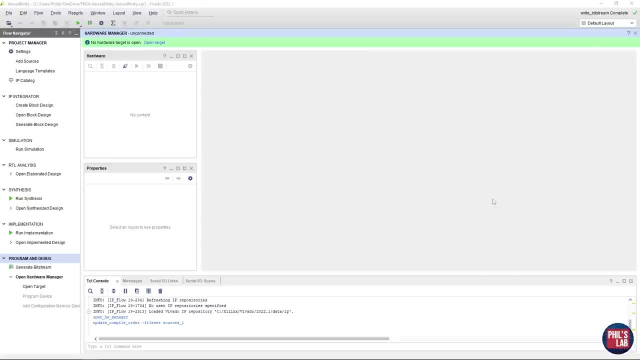 Afterwards I'll also show you how to configure the configuration memory so the FPGA gets reconfigured every time you power up the board, Because in this way, every time you unplug power or you reset the board, the FPGA will not be configured. 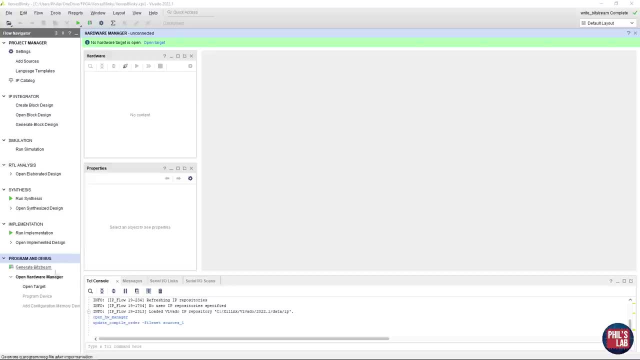 First of all, where you can do this is go to Open Hardware Manager on the bottom left. I've connected my board with my USB-C cable, which powers the board and also provides my debug interface via the USB JTAG converter. Then Open Target Auto Connect and we can see. 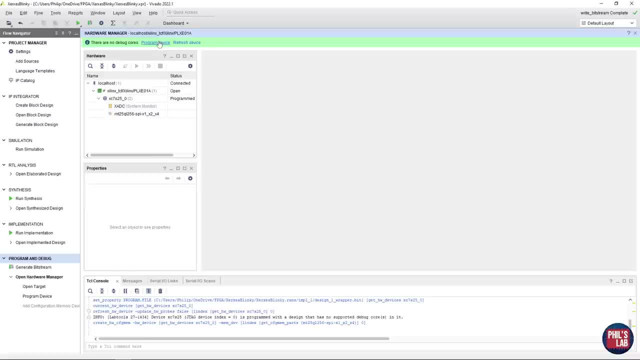 my device, my FPGA, is discovered. I can then click on the top on Program Device and it should automatically select the right bitstream for you and simply click Program. And this should be very quick. And now let's move over to the different camera view to see. 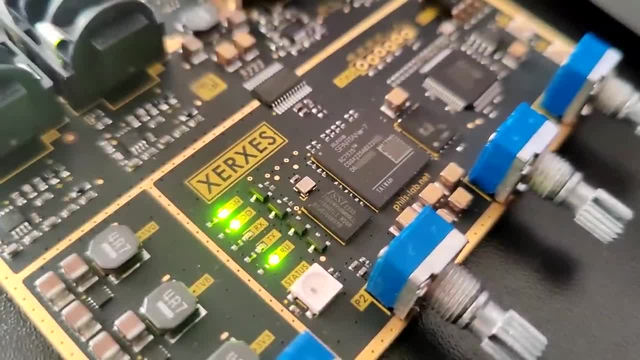 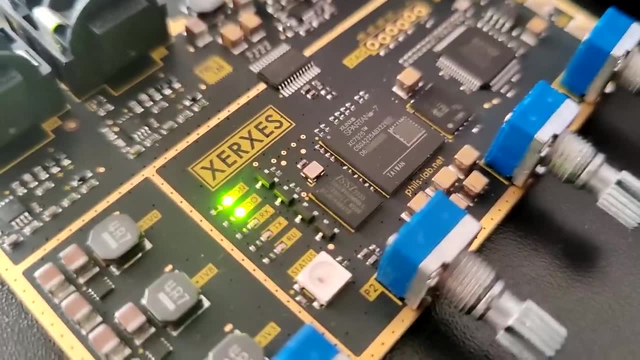 that our logic is now running. We now flashed our bitstream to the FPGA directly, so not using the configuration memory. I'll show you that afterwards And we can really see our HDL design is now running. You can see below the On LED, the first LED, there's the Do or Done LED. 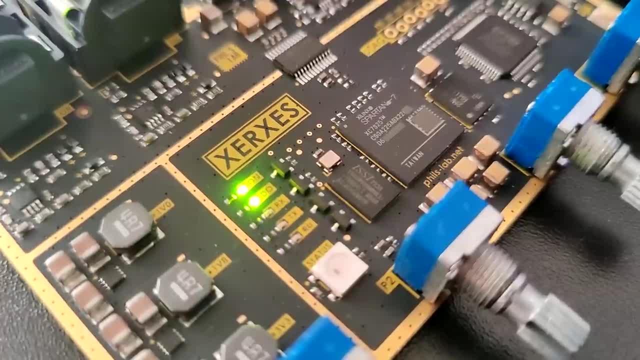 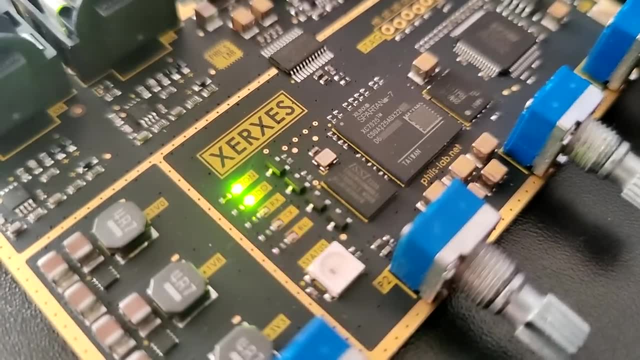 which indicates that the programming or the flashing of our FPGA was successful. Right at the bottom is our Use LED, which I've just called a Run LED RU for now, and that's flashing with the on time we specified. On the right side of the board we have our DIP switches and in position one 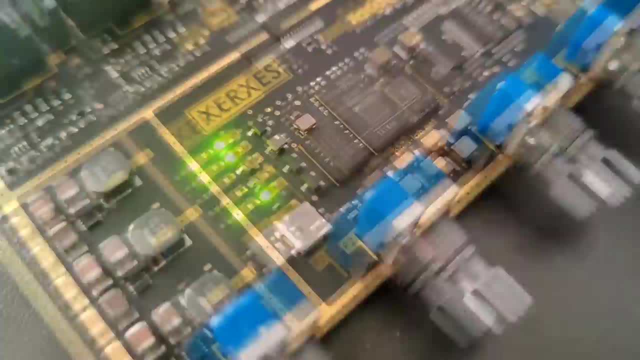 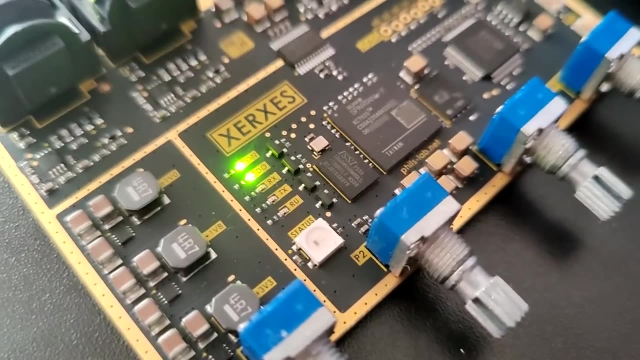 this is our DIP switch. we assigned is currently in the low position and therefore the LED is a longer on time. Now if I adjust the DIP switch in the top position you can see the Run LED is now flashing double the frequency half the on time, as we set in our HDL. We can, of course, 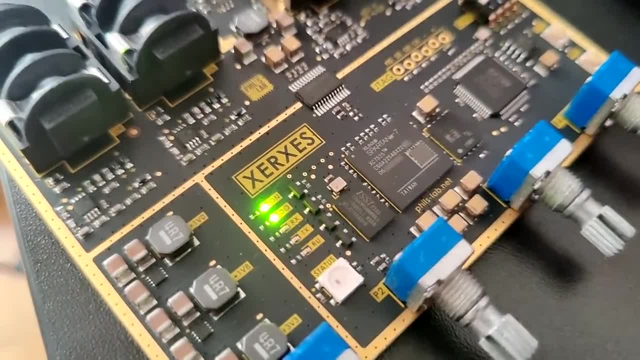 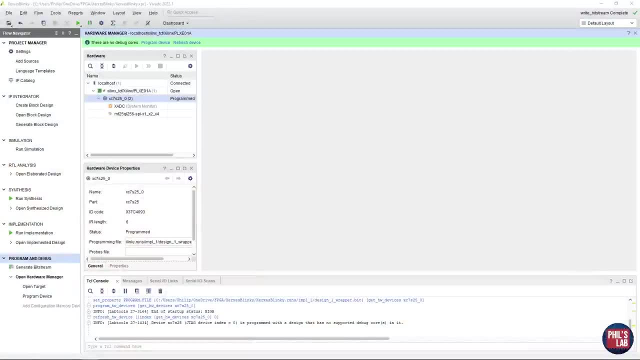 toggle that back down again and our LED now turns on for longer and off for longer. This looks like our HDL, and our implementation is working straight away. As we said previously, this is all great. We have our blinky logic running. We now have to now write a bitstream. 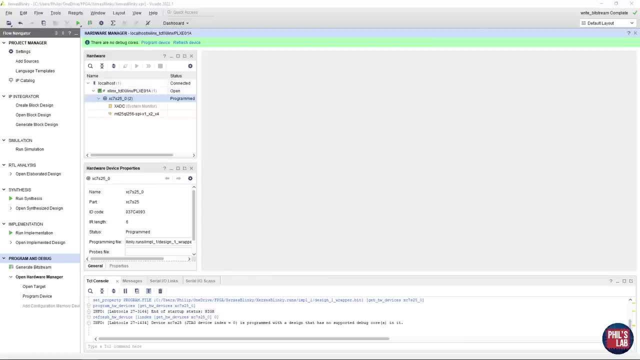 and reconfigure the device, But this is volatile, meaning every time we unplug or reset the board we have to flash our bitstream. What we can do is create a memory configuration file for our memory configuration device, where the appropriate boot settings can then reconfigure the FPGA on. 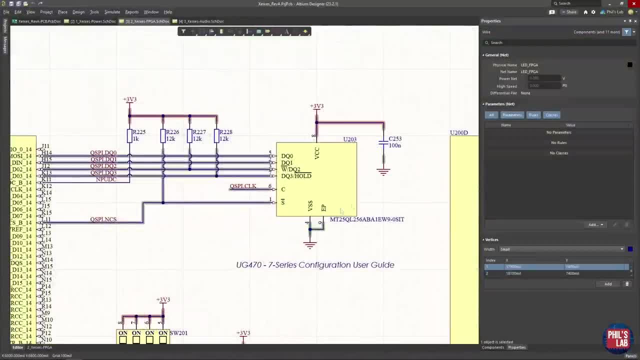 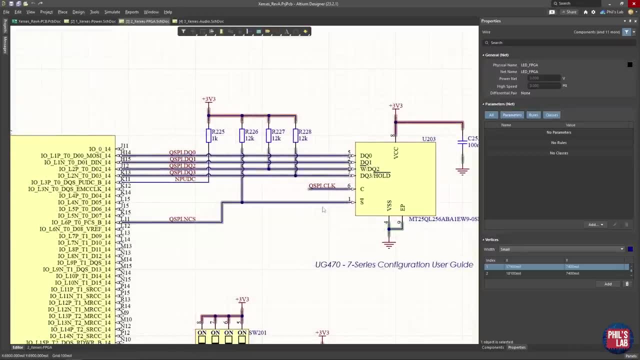 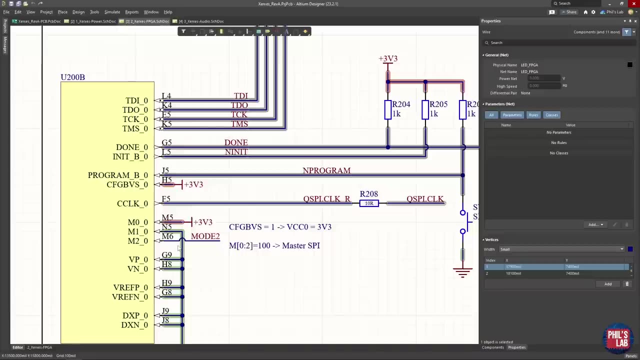 startup. Going to the schematic, the configuration memory device I'm using is this Micron MT25QL, which has a capacity of 256 megabits, and it's connected to the FPGA- pretty much a point-to-point connection That, in addition with these M0,, M1, and M2 pins, determine the boot configuration. 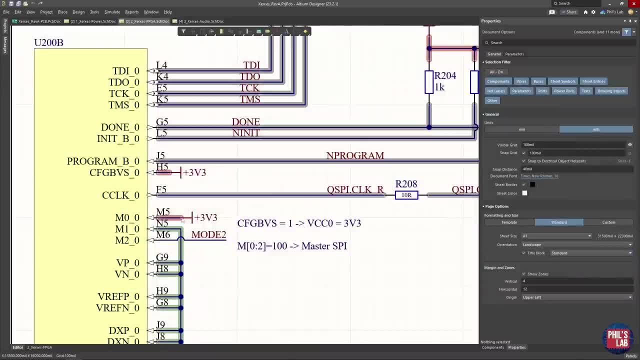 or the boot mode. very simply, speaking of the FPGA, If we have M0 high, M1 low and we can toggle mode two, we can have our FPGA either boot just via JTAG or pull the bitstream, so to speak, from our configuration memory, This mode two. 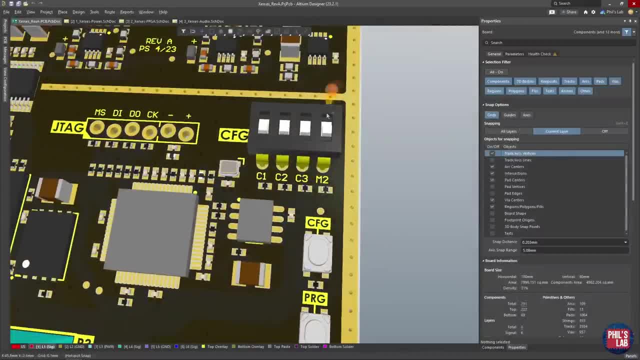 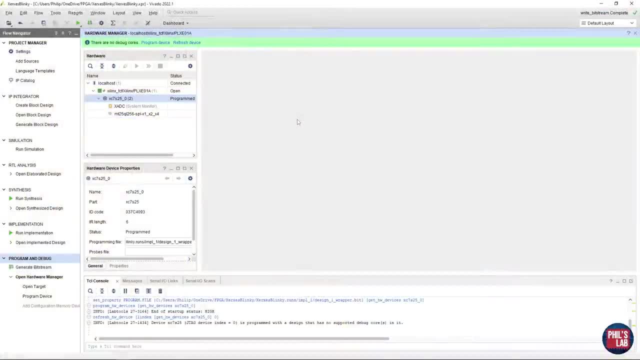 configuration pin. I can pull high or low on this array of DIP switches on the right side of the board. Let's now see how to generate the configuration memory file in Vivado and then how to flash that onto the configuration memory. After we've generated the bitstream, go to the top tools. generate memory configuration file. 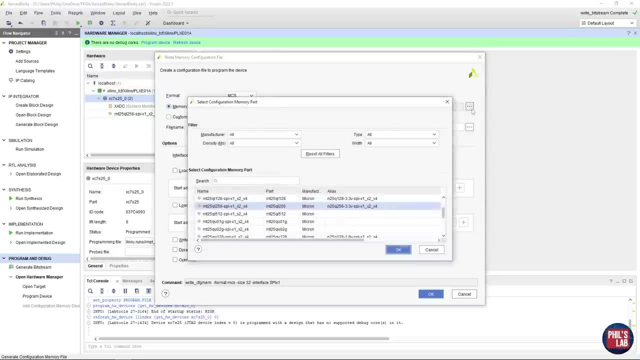 we need to choose a memory part, so I'll click on memory part. On the dots on the right-hand side you can choose the right part you used for your design. There are very specific parts you need to choose for your design and that's given in a user guide by AMD Xilinx. But this is the part. 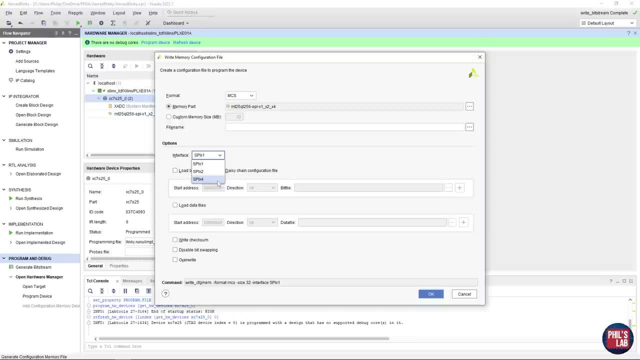 I'm using, so I'll select that The interface is QSPI, so SPI times four. We can give this a specific file name. For example, I'll just call it Xerxes Blinky, MemConfig, and it's an MCS file. 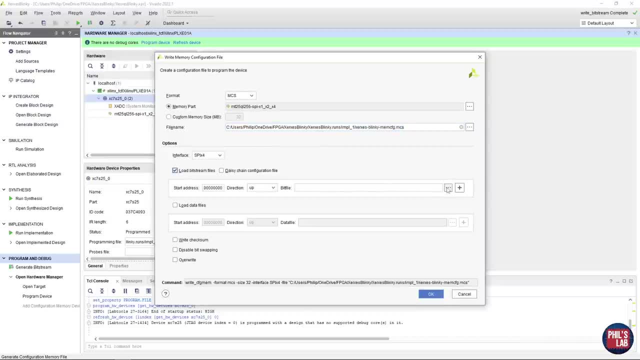 I would like to load the bitstream files, so I'll need to check this and I need to select my bit file, which is the one we previously used. I'm going to click on the bitstream file and I'm going to click on the bitstream file and I'm going to click on the bitstream file, which is the one we. 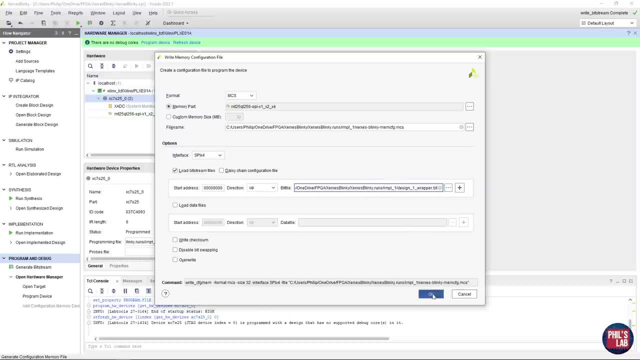 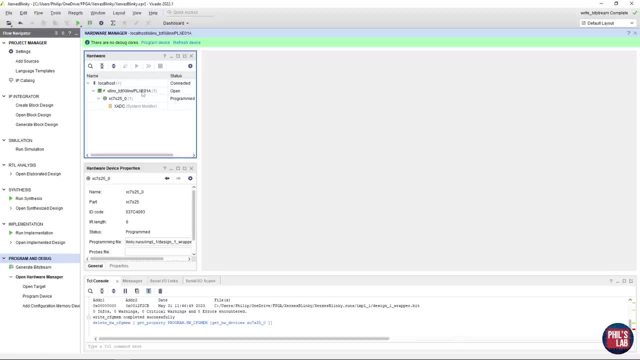 previously programmed the FPGA with. The rest you can leave as standard and simply click OK. Then it should come up with a success message To then flash the configuration memory we need to add in the hardware manager. after we've already connected to our FPGA, We can right-click. 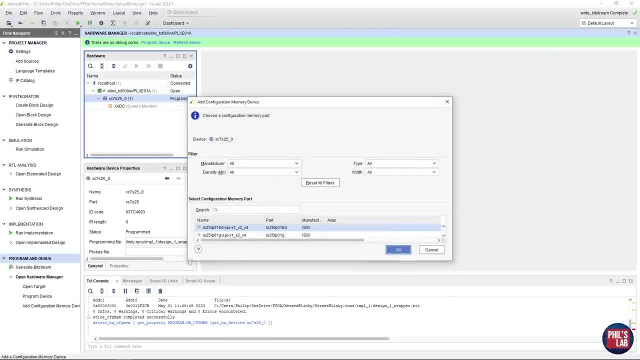 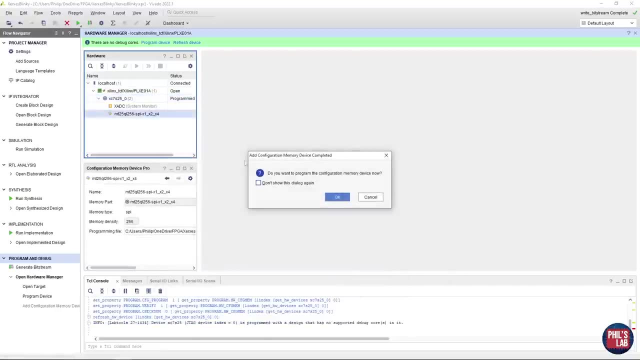 on this and click on add configuration memory device and we need to choose the device we are connected on our board. In my case this was the MT25QL256, so click on that and this should add it to the device. Now it immediately asks us if we want to program the configuration memory device. 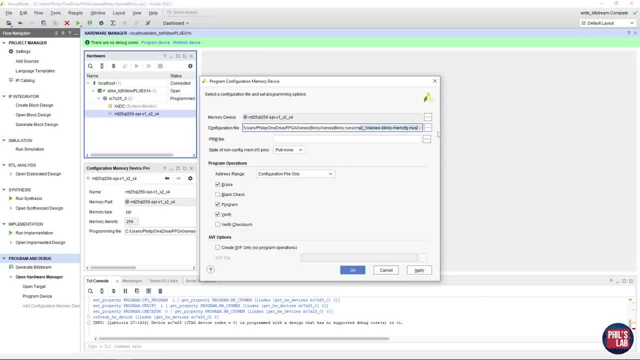 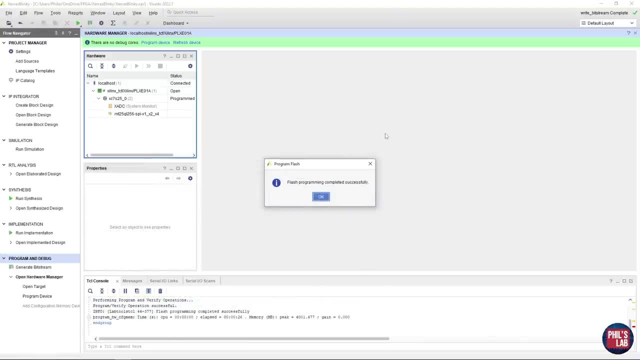 Click on OK, It should automatically find the MCS file you defined. You can leave everything else as standard and click OK. This should take a minute or two to do, and then the flash should be programmed successfully. If you've already added the flash memory to your device, all you have to do is 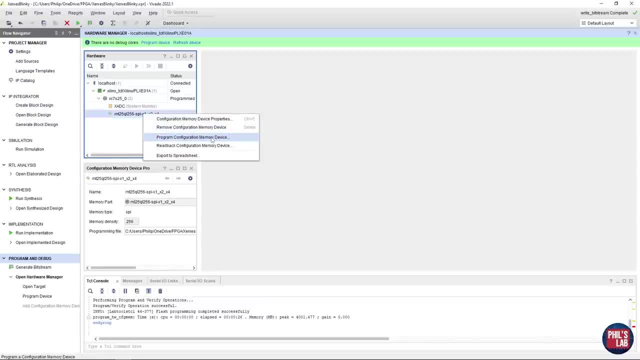 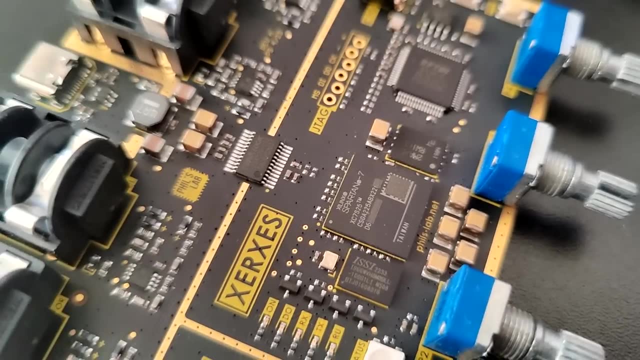 right-click and then program configuration memory device. and that's what we just did. We've now programmed the configuration memory device, this Micron MT25QL part, with the bitstream configuration. So if we have the right mode- setting the M2, in the low position- then